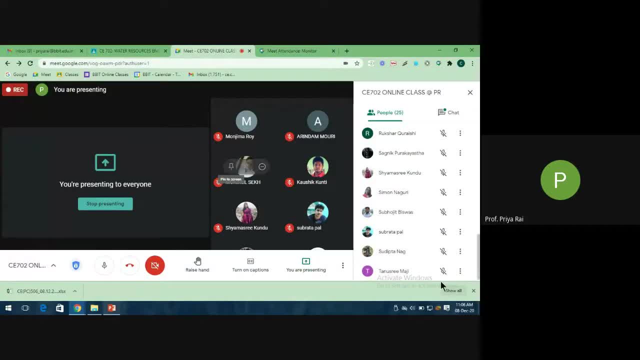 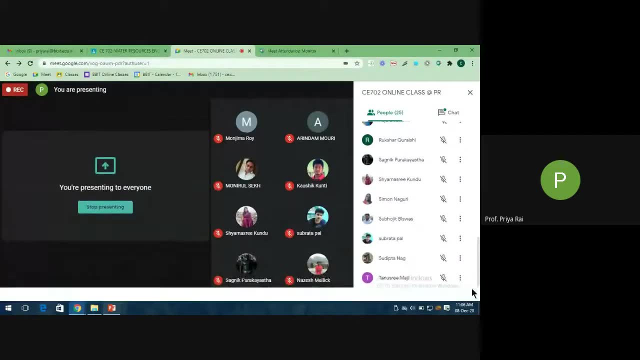 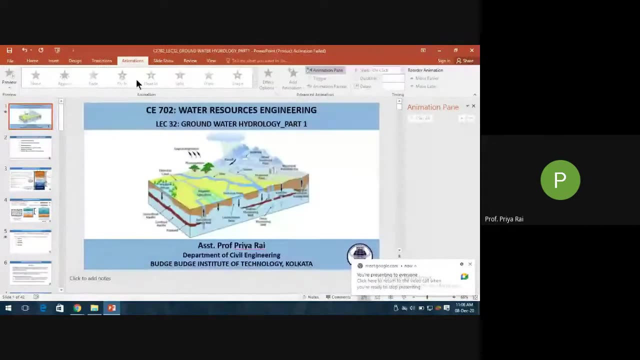 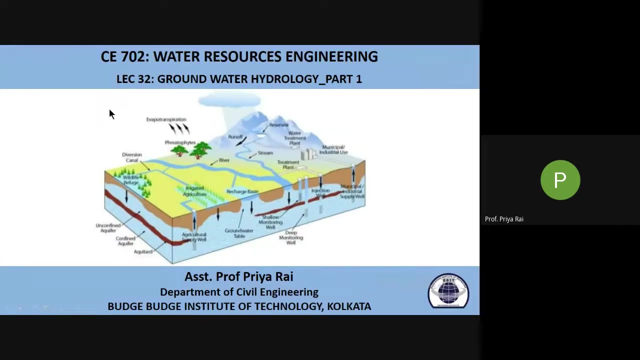 Okay, let us start. So, good morning everyone. This is our water resource engineering class. Okay, and today we will learn new module in your water resource engineering. Okay, that is the groundwater hydrology. Okay, now, what are the? 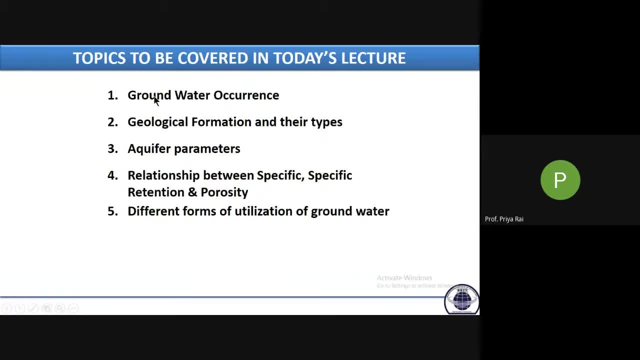 topics that we will learn today. We will see. what do we understand by the groundwater? Where does it occurs? Okay, how it occurs. What are the different parameters that we have to consider? What are the geological formation- This is very important for your short notes purpose, Okay, geological formation- and the types. And, based on it, only there is one type of geological form, which is your aquifer, which is known as aquifer. So what are the parameters of this aquifer? We will learn that also And we will try to 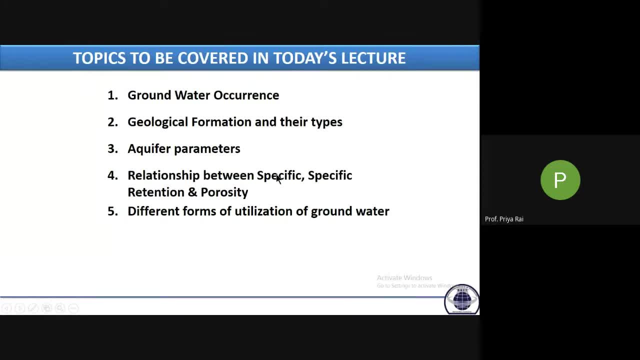 solve. what is it? We will try to build a relationship between derive, the relationship between specific yield- Okay, it will be yield- Specific yield, retention and porosity. These three are aquifer parameters. Okay, Now we will see the relationship between these three parameters. And, lastly, we will see what are the different forms of utilization of groundwater. That means 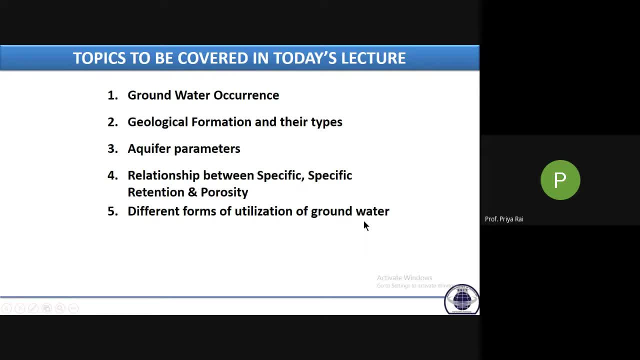 how can you use groundwater, In how many forms? Okay, This is what This is. what are the groundwater sources? In which form does it exist Beneath the soil or beneath the earth? in which form does your groundwater exist? Okay, And how we are using. 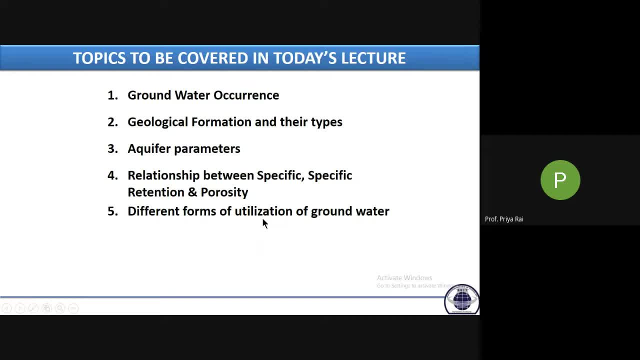 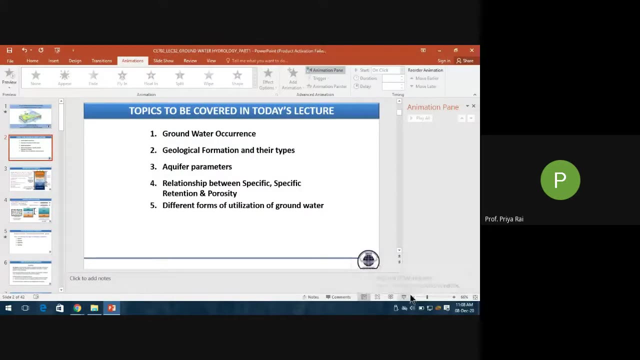 How will we extract water from that groundwater source, In which procedure, which manner or different forms? Okay, We will see that also today. So we will see that also. Okay, So groundwater is what It is: the water which exists in the pore spaces. Okay, 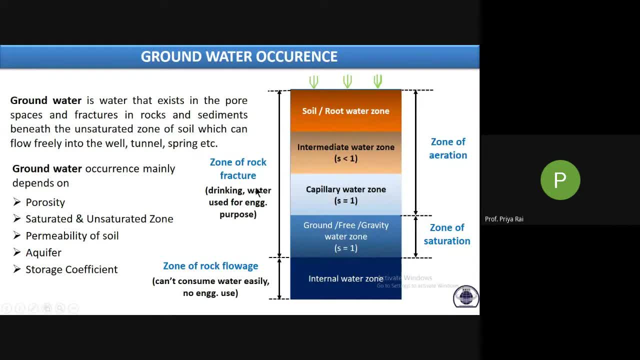 That means this soil structure has been formed Beneath the soil. we will divide this into many zones. Okay, You will not get water immediately. Suppose this is the earth surface Immediately. if you dig beneath the earth surface, you will not get water. Okay, 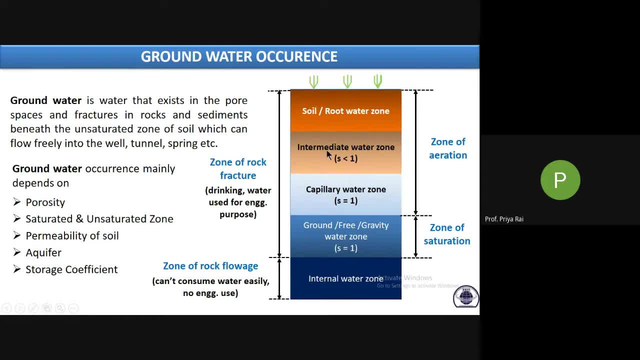 You have to, It is not visible. Okay, You have to go much deeper, then you will get water. so now, amount of the water which is stored inside this earth, inside the soil, within this earth. how much ground water is there on which thing? 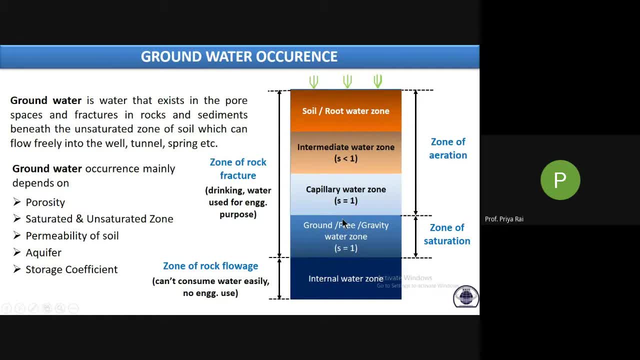 depends actually where your water is stored, where your water stores what is your earth? earth is a combination of what voids and solids. this is a structure okay. so where as the voids are there, the more capacity to store there is okay. so that is why look. 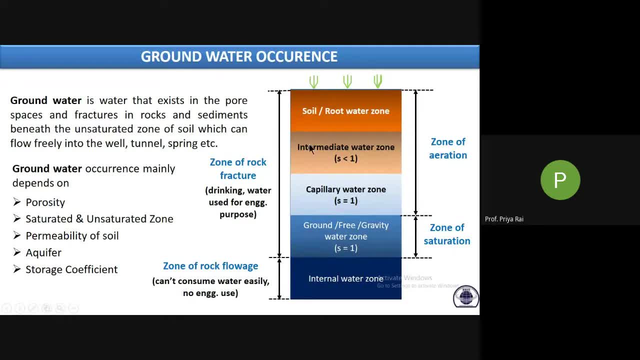 here I have said it is stored in where. in the spiced means whatever spiced the space here your water will store top in the spiced and in fractures. Islamic fractures means there will be a rock under it which will be very heavy. there is an impenetrable streaked. 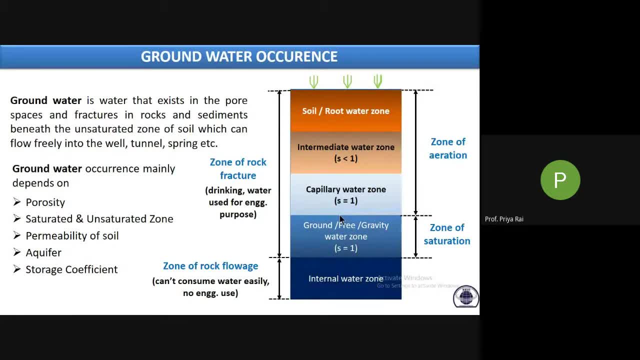 rock in between it. if it comes to a fracture, What happens? A gap is creating. So as soon as 80 minutes we come here, it will take us to the half. in mean time, the we have already seen that in our hydrology classes that 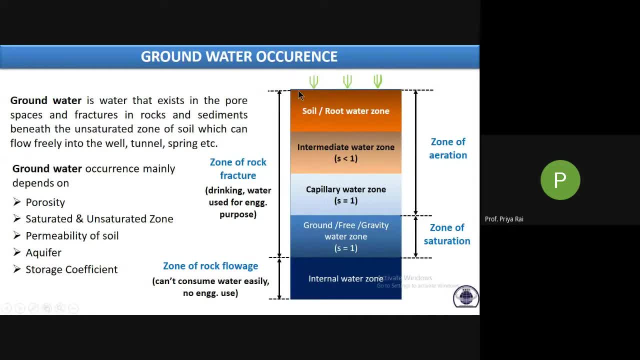 the rain water is infiltrated and ultimately it goes down to the ground water. only right, because of infiltration, this water is getting stored down. so how is it going? it depends upon the fractures. your pores are big or small. it depends upon if it is a permeable type of soil or an impermeable type of soil. 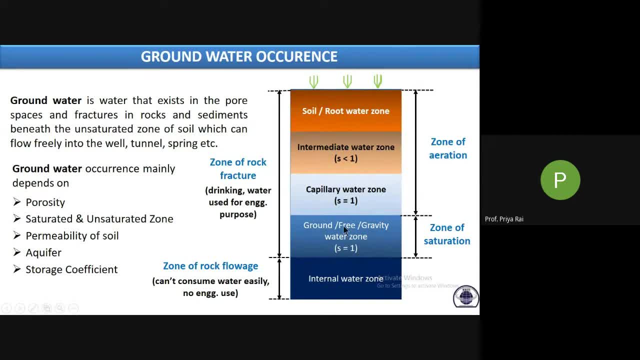 it also depends upon the amount of ground water stored in it. obviously, what is permeable? there are two terms. one is porosity and another is permeability. porosity means how much voids are there. the more voids there are, any object is porous. for example, if you bring a sponge and a wood, 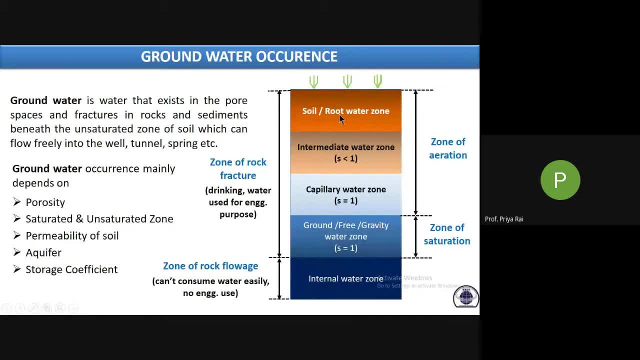 which one is more porous. obviously, in a sponge the water will be absorbed more, because the water will absorb more because there is more porosity. so porosity again depends upon the size. what is the aggregate of the soil? what is the nature of the soil? 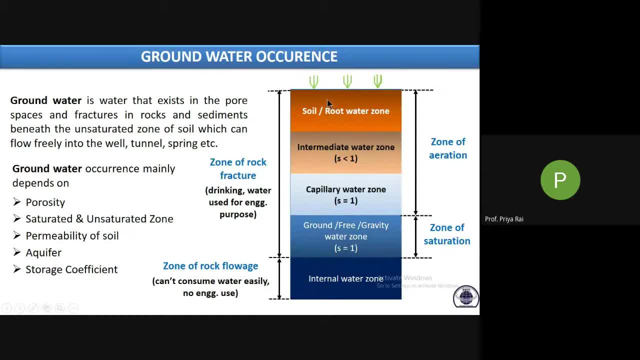 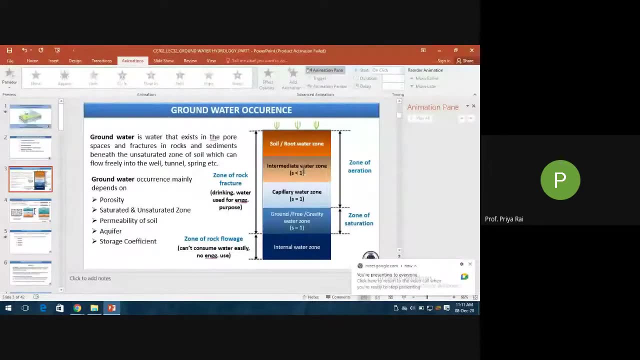 what is the type of soil? it depends upon the porosity. also, permeability- now this is a porous soil, but it is not permeable- means you can store water in it, but it is not permeable. what does permeability mean? permeability means downward movement. 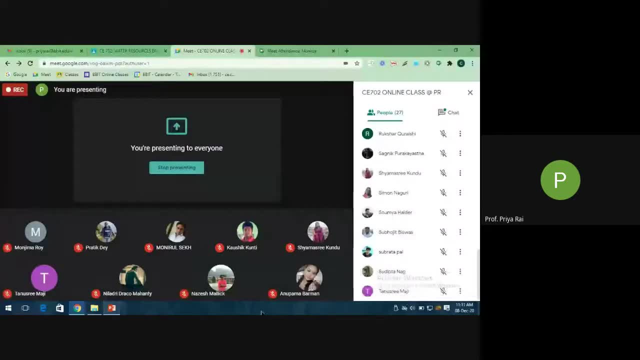 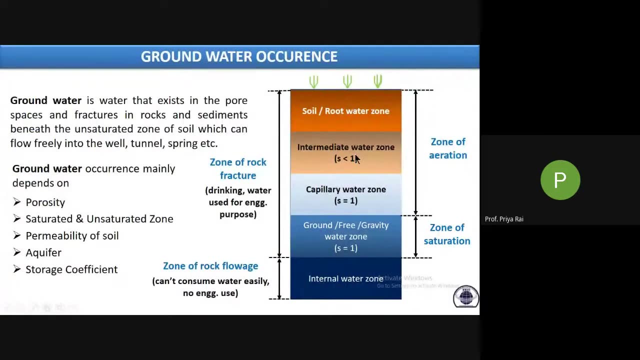 ok, how will it move? permeable means how will it flow downward, how are we permeating the water? so if there is more permeability, then it will transfer quickly. it will move downward quickly. it will be stored in the ground water. ok, some soils are porous. 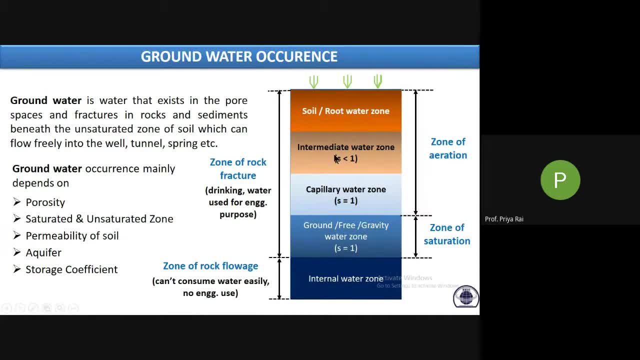 they can hold the water, but they cannot transmit the water. this also happens in some soils. ok, in some soils they are both permeable and porous. they can hold as well as they can transmit water. ok, so based on such type only, your ground water sources also vary. 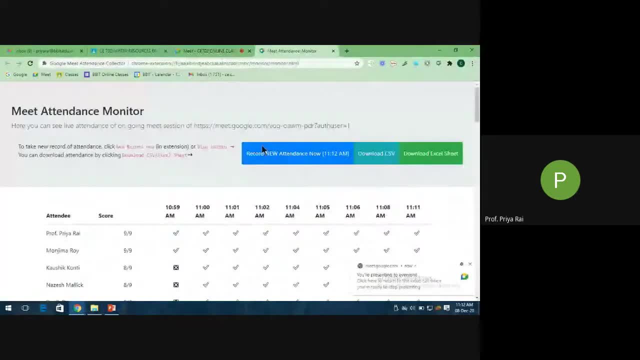 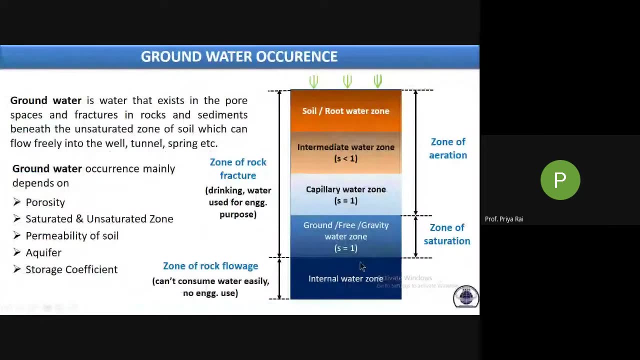 ok, so so these are the different reasons. what is it first comes your root water zone. what happens from here? the water that will be used for the roots will be taken. who is taking the water? the roots are being taken here. we cannot use that water. 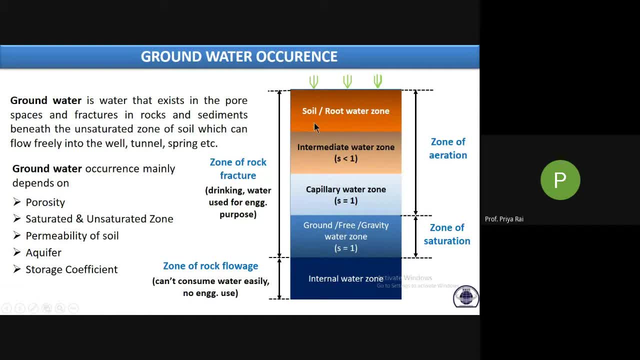 means we cannot get the amount of discharge from the bottom. ok, so what is the second intermediate? and this is not saturated, this is not fully saturated. some of its pores are some of its pores. actually, what is your soil made of? it is comprising of void. 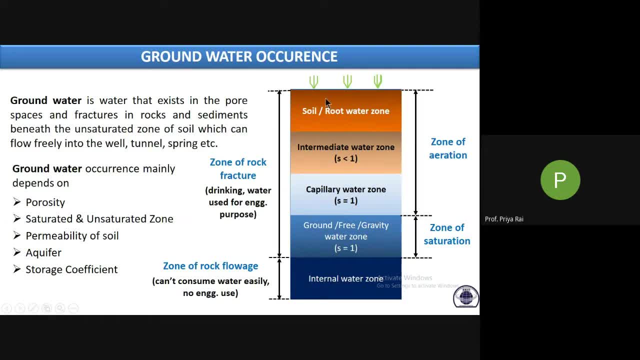 and solid particles. ok, so in the void, total void. if it is fully, I mean total, all the voids. if the water is completely frozen, I mean filled, then it is fully saturated. ok, so this is not saturated. intermediate is also not saturated. that is why saturation, degree of saturation is less than 1. 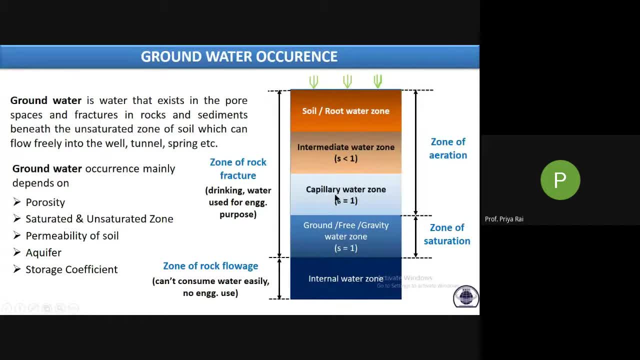 now what is in capillary? in capillary is s. s is equals to 1 means this is also coming under saturation, ok, but here water is in capillary motion means this is upward. capillary means it is rising above. water will go upward because of the 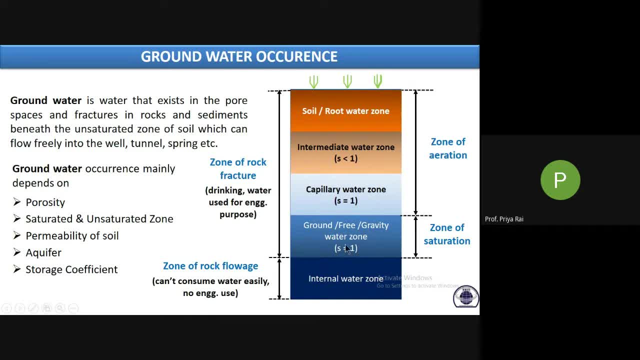 capillary motion because of that. ok, and this is what this is: the groundwater free or gravity water zone. ok, here, what is there? your whole flow will be means water will be here. all the voids are full, it is fully saturated with water. ok, so see what is this. 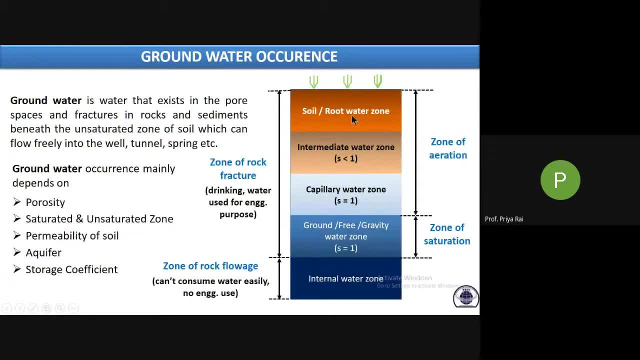 this is here zone of aeration. here some voids are filled with water, some voids are filled with air, ok. here zone of saturation means everything is filled with water, all the voids are filled with water, ok. and from this region to this region only we will get water. 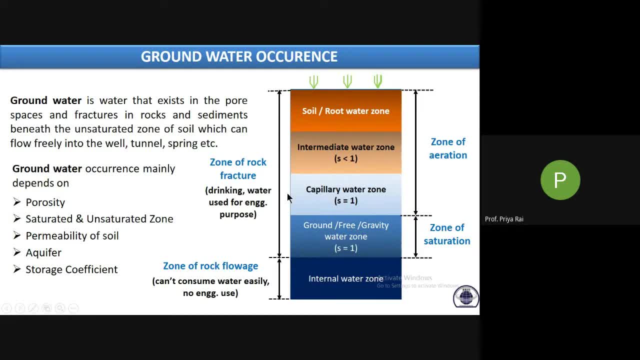 for engineering purpose or drinking water. we call it water. ok, so from where we get drinking water we can get only till this region, and there will be more down there. there will be more water, but we cannot extract that. ok, so that is called zone of rock flow. 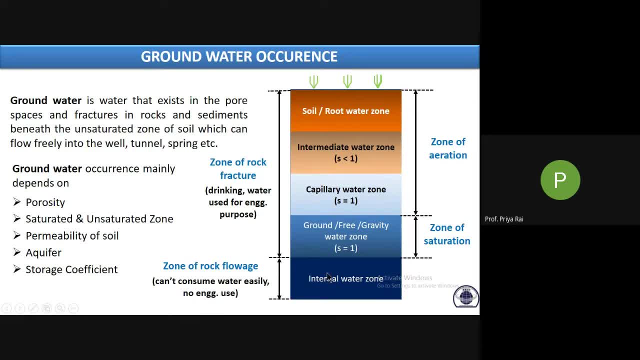 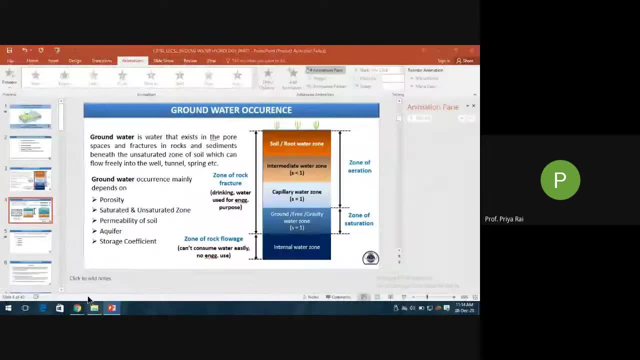 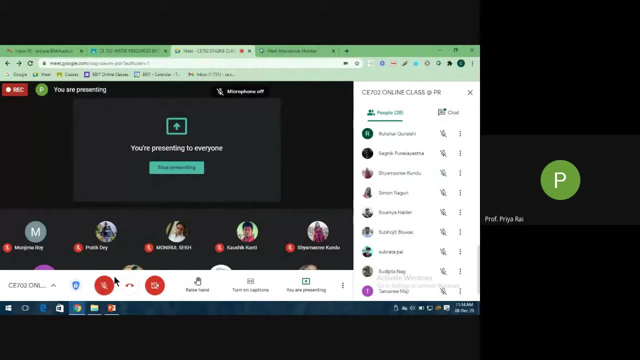 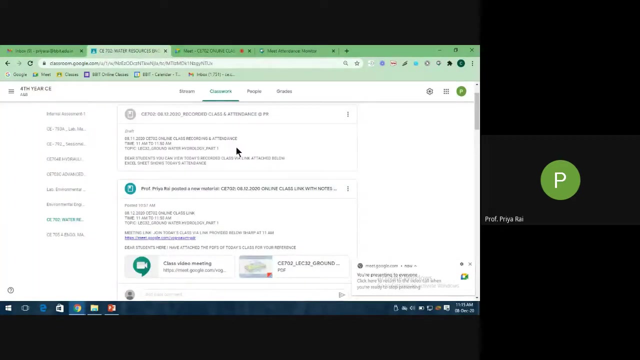 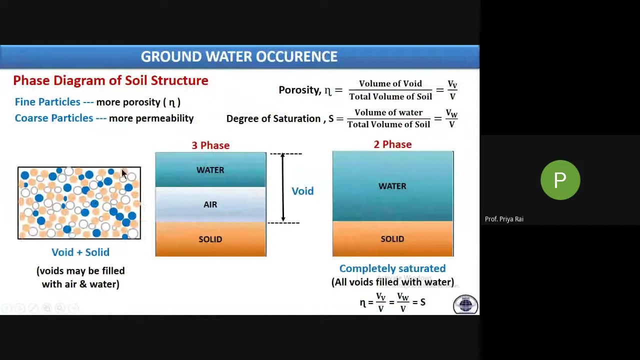 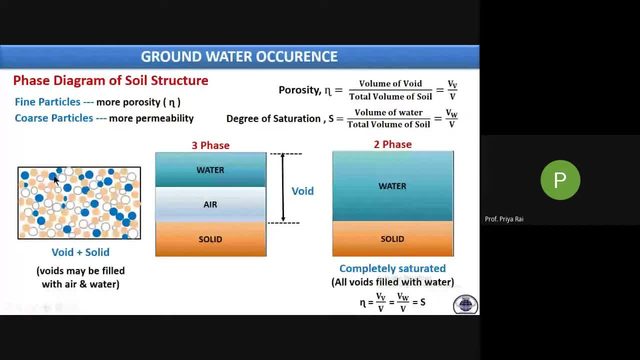 This red is the desired solid particles, this blue is water and this white is the desired air. The total blue and white particles are the void particles And the solid particles are red. Some of the voids are filled with water and some of the voids are filled with air. 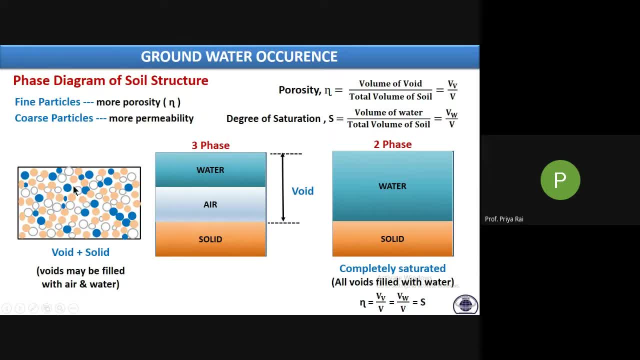 In this case it is not fully saturated because some of the voids are filled with air. That means the water has not yet gone there. So we can define it in three phases. The three-phase diagram of the soil structure. This total is a void and this is solid. 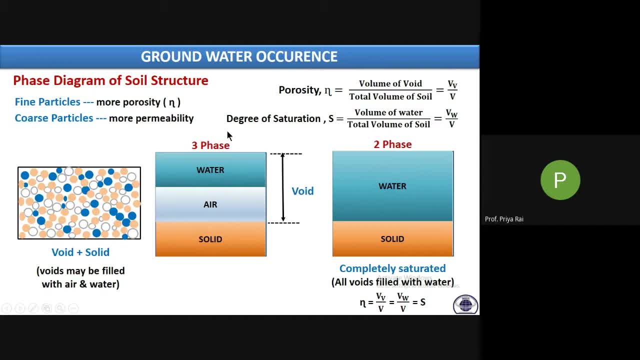 If there is water and air, then it is a three-phase. What happens in the two-phase? If it is fully saturated, that is, the voids are filled with water, then it is completely saturated. Now, what is porosity? 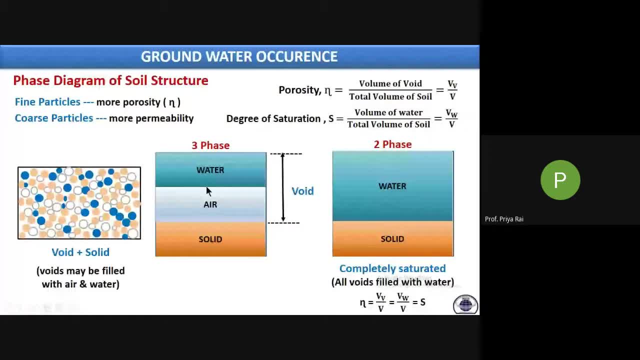 What do we call porosity? How many voids are there in porosity? We are taking a certain volume of soil. It has voids and solid particles. So what is the total volume? What is the percentage of voids in the soil? 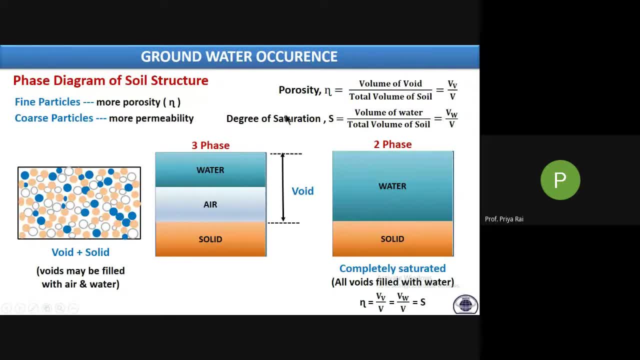 That is the porosity And what is your saturation? How much water has been saturated in the voids? We will take the volume of the amount of voids that has been filled with water. We will take the volume of the voids that have been filled with water. 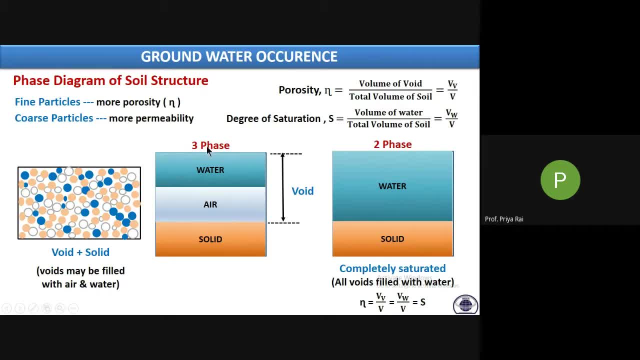 That is Vw and the total volume of the soil. If the total volume is V, then it is V. So if it is completely saturated, then we can say that the total volume of the voids is Vb And the total volume of the water if it is fully saturated, if it is Vw. 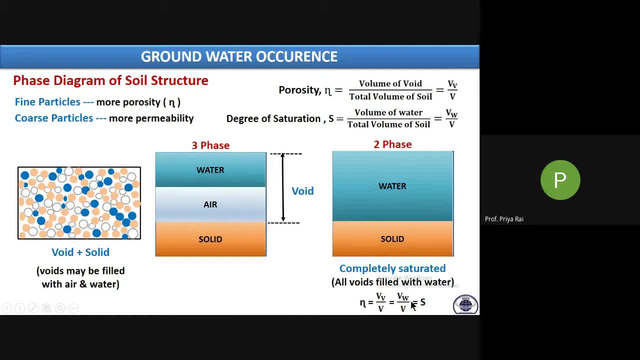 then we can write: in that case, porosity is equal to S. We can say from this equation: When will it happen? When all the voids will be filled with your water. So this is the phase diagram of the soil structure. It depends on this how much groundwater can be stored. 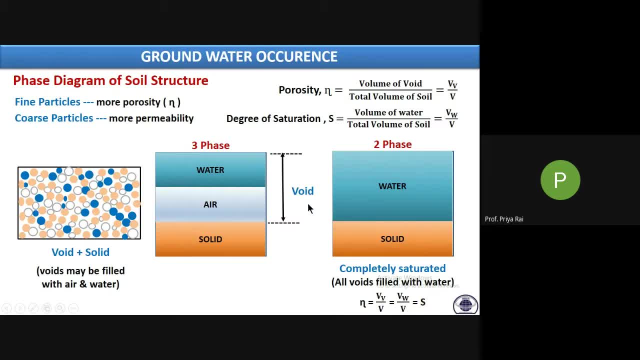 Different types of soil. That is why we see the structure of the soil. It depends on the structure of the soil that how much capacity you have, How much amount of water we can drain out from such type of soil. It is storing at one place. 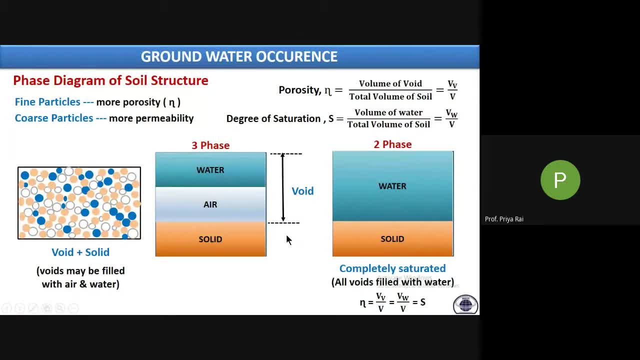 But we have stored the same amount of water. We have to take out the water from the soil, Whether in form of tube well, whether in form of open well. So depending upon the type of soil structure, only how much amount of groundwater comes, how much discharge comes, it varies. 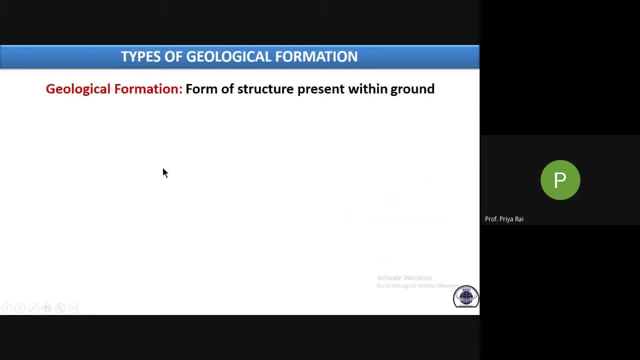 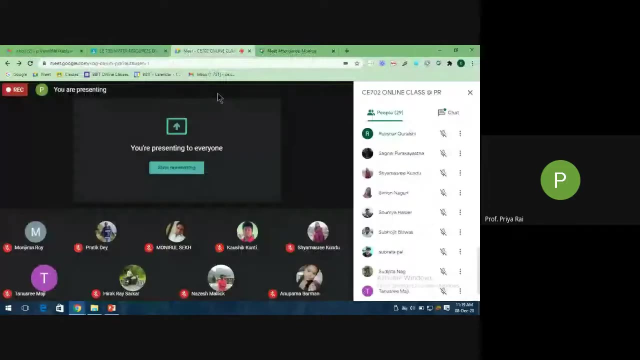 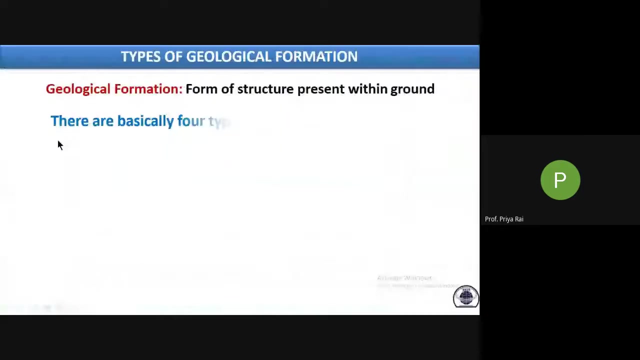 So now comes the geological formation, Which is what The forms of the structure present within the ground. So what are they? There are basically four types. One of them is called the important one. This is your aquifer. So one is the aquifer. 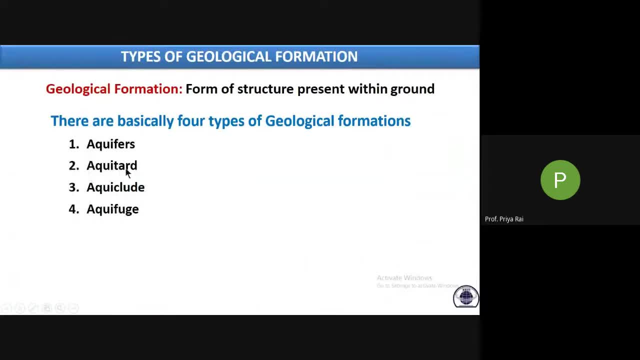 The other is the aquitard, the aquifluid and the aquifers. All of these have short nodes. So if we talk about the simplest one, We can call the aquifer the transfer. Okay, We can call the aquitard the tired structure. 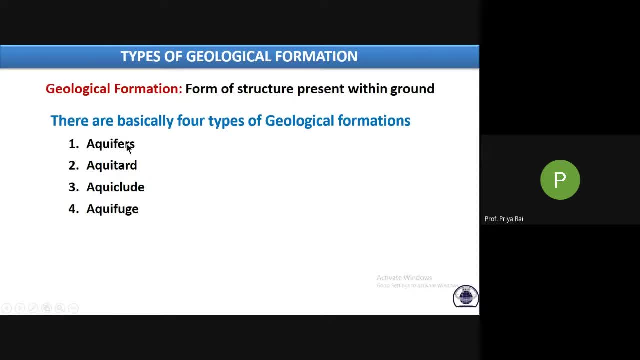 The structure which can be transferred is called the aquifer. The structure which is tired means it will transfer slowly. It will do it. but it will do it slowly. What transfer? What we are learning? We are learning the groundwater Right. So the groundwater which can be transferred through that medium is known as the aquifer. 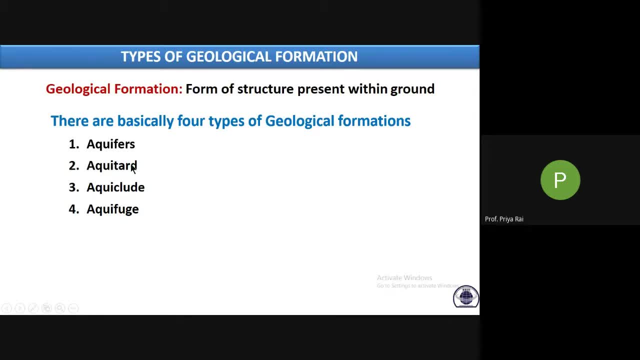 Groundwater which can be transferred, but in a slow way. In a slow manner. It is called the aquitard because it is tired. Okay, Aquifluid means it includes, Only it can include. Okay, It means it does not transfer. 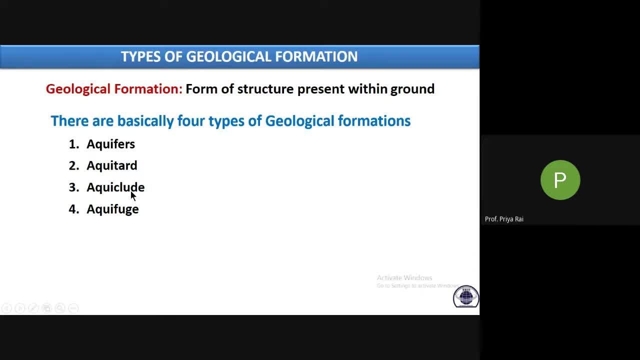 It only stores the water in itself, But the water cannot be transferred through it. Groundwater, Okay, And the aquifuse means it is confused, Totally confused. It means it does not store the water, but it does not transfer the water. 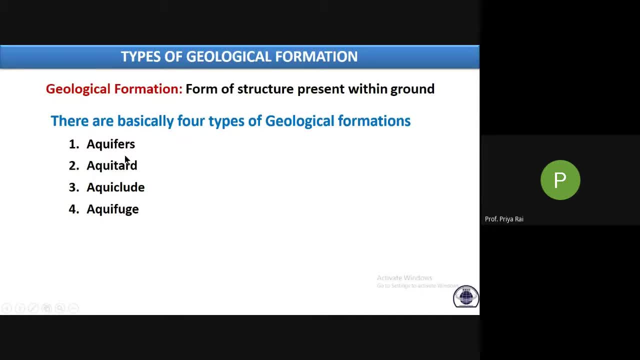 Okay, So basically, these are what It depends upon: the type of the soil, Nature of the soil, Who will be called aquifer, Who will be called aquitard, Who will be called aquifluid, Who will be called aquifuse. 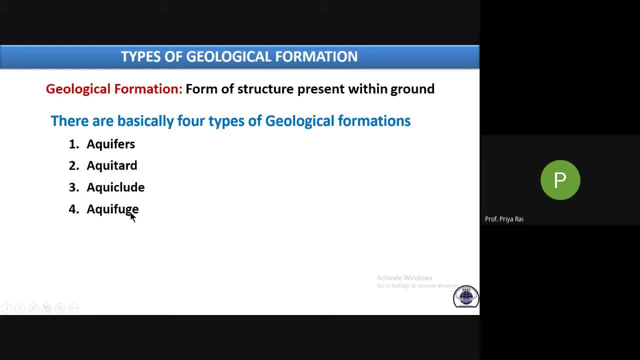 Okay, So see, We said aquifer. This is all a theory. You have to see a little. If we explain in detail, then see a diagram. This is one type of structure. Okay, What is this? Will there be water in it? 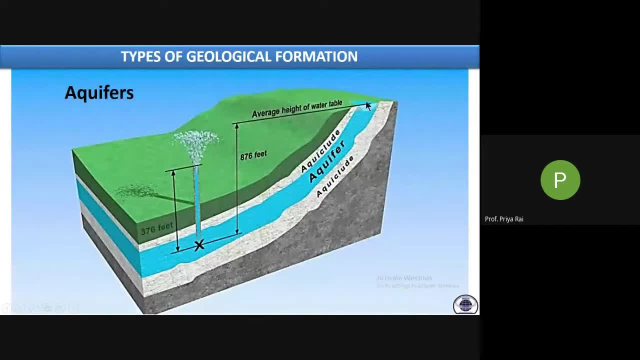 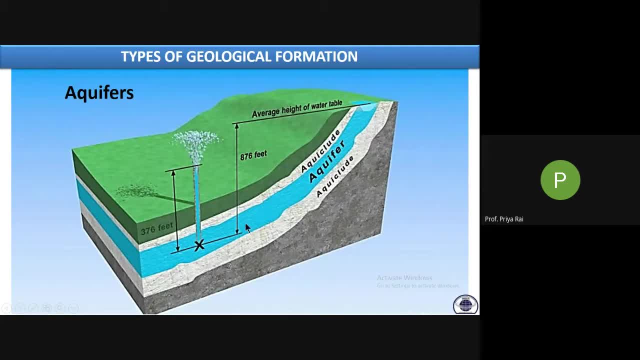 It is soil. So what is it? It is soil Okay. So what is it? It is soil Okay. So what is it? It is soil. It is soil Okay. So what is it? It is soil Okay. 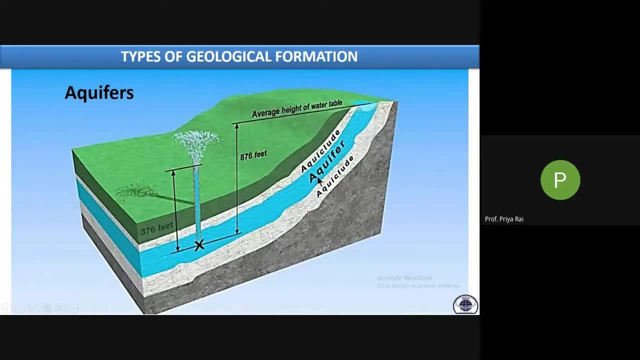 So this is called aquifer, Okay, So what is the example here? Which it can hold as well as transfer? What is the nature of soil? What can it do? Gravel, Which is very big gravel, Okay. What happens to them? 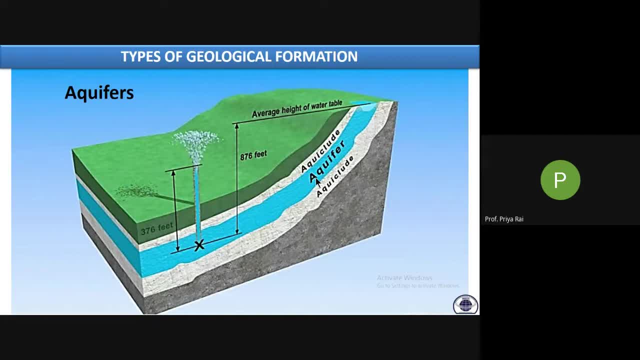 Particle size, That is, there are many voids. What does that mean? More voids means more soil saplings. So what does that mean? Porosity means it can absorb more water. right, So it can absorb more amount of water. 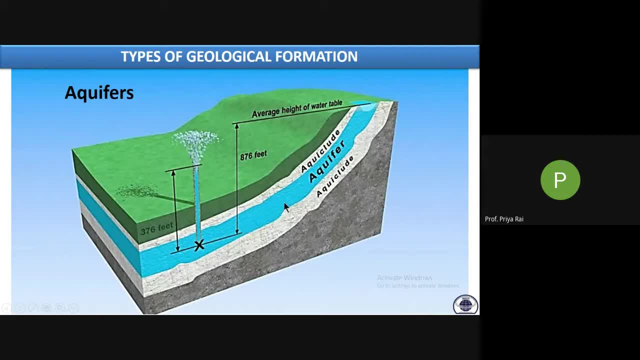 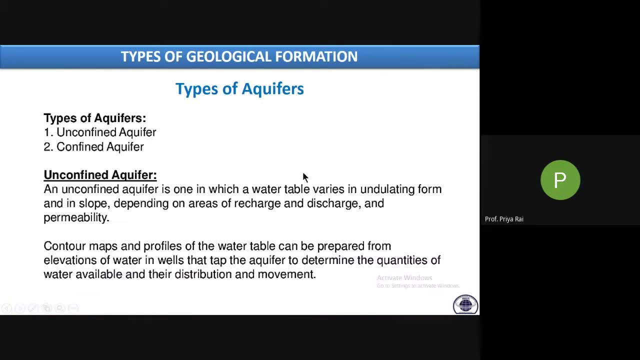 as well as the permeability here is also very good. It means it can also transfer the water. Water can flow also, Okay, so this is called aquifer. okay, Now in the second one, you guys, under this aquifer comes types of aquifer. 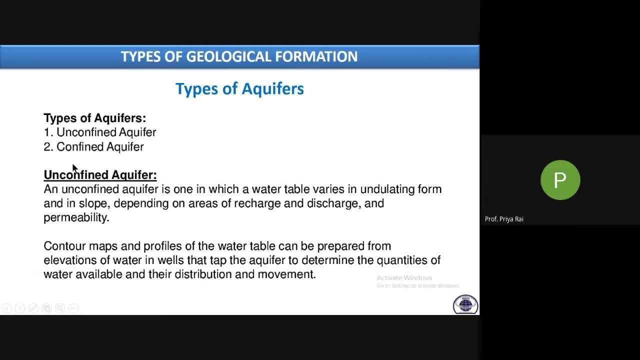 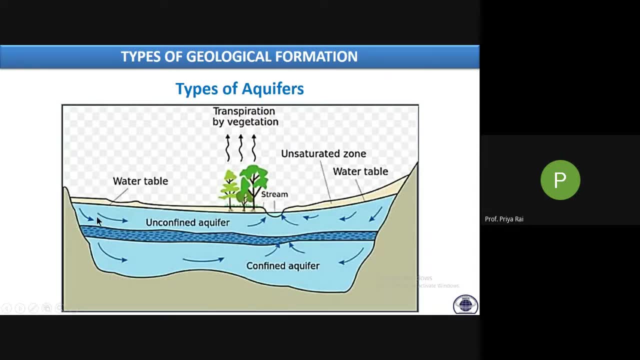 What comes? mainly Confined aquifer and the other one is purged aquifer. Okay, so what is a confined aquifer? See, these two are aquifers. Don't think that this blue color means water is flowing here. No, it is not water, okay. 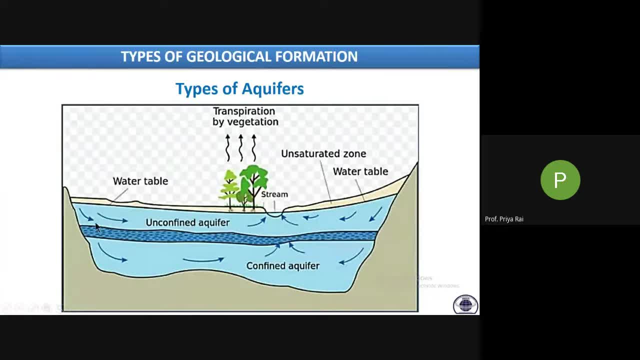 Actually, what is this one? This one is your soil, any of the soil voids which is filled with water. okay, We are taking water from the same water. we are taking groundwater water. okay, We are taking water in the form of groundwater. 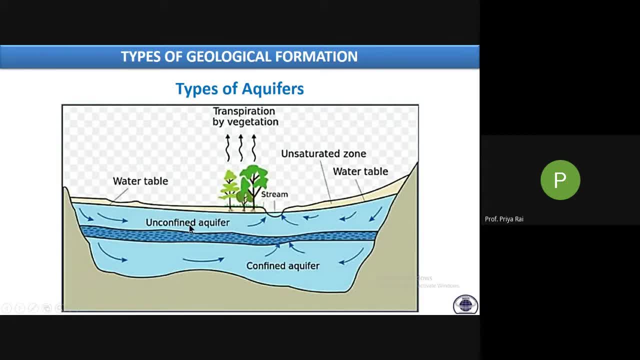 Okay, it can also be done through wells, it can also be done through tubules, it also can also be done throughشرps. it can also be done through crushed clay. Okay. So confined means Unconfined, means that its one layer. 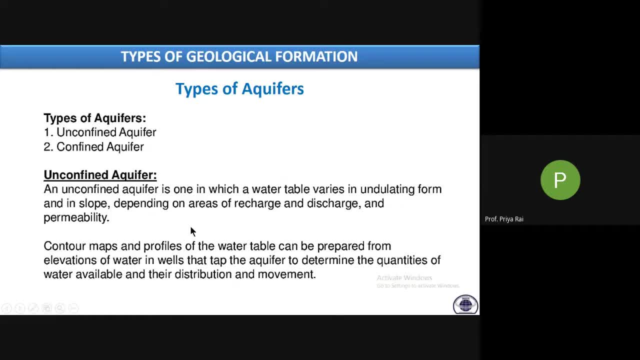 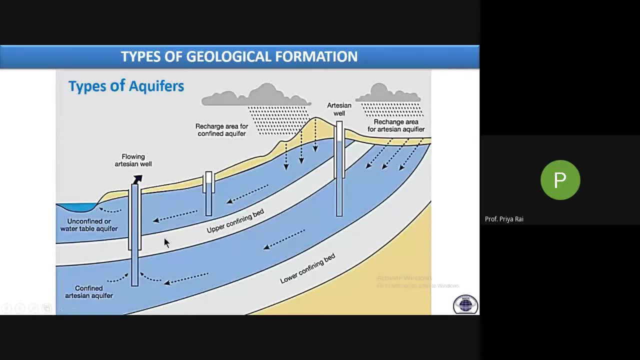 what do we want in it? One layer should be impermeable. okay, See this one. What is this? This is your impermeable type of layer. Okay, Here, water will not go down or it will not even transfer. It will neither hold nor transfer. 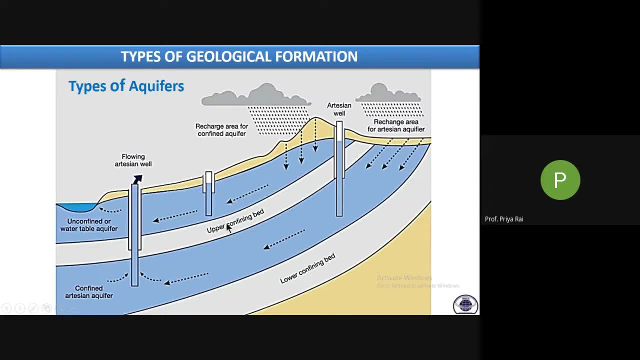 This is impermeable. It is hard strata, hard rock. Okay, What does the query mean? What I have studied in water flow, What are water keeping in water? The upper layer is soft and the bottom layer is permeable. 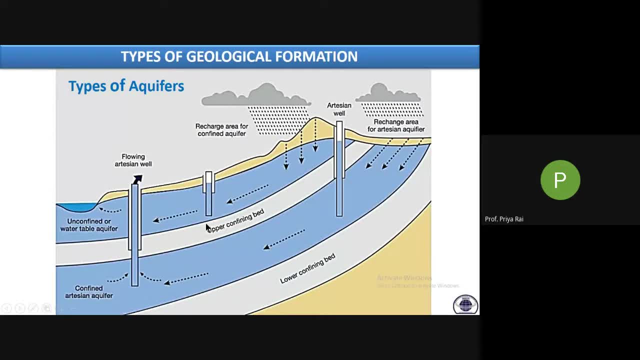 One layer is permeable and the other is impermeable. This is called unconfined. This is also impermeable, and this is also impermeable. There is a layer between the two impermeable layers. This is your confined aquifer. 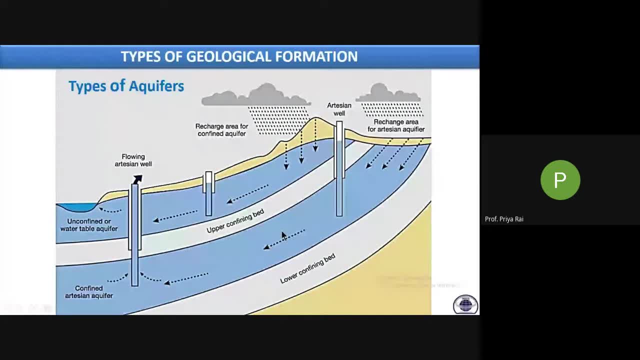 Okay, Tell me which one will have more pressure. Which one will have more pressure? We will dug a well here, and we will dug a well here. Which one will have more pressure? Which one will have more discharge, This one or this one? 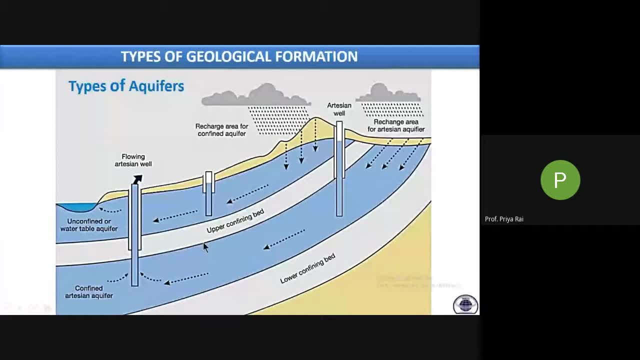 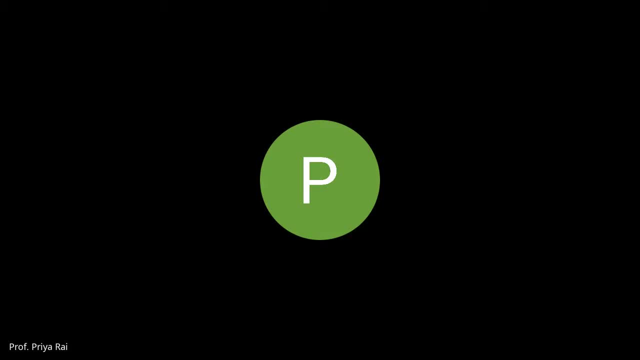 This one. Take it one more. Yes, because this one has more pressure. This one, Because there is pressure coming from both sides. Right, There is impermeable on both sides, And here is the hyper static pressure, Which means the pressure of the normal water table. 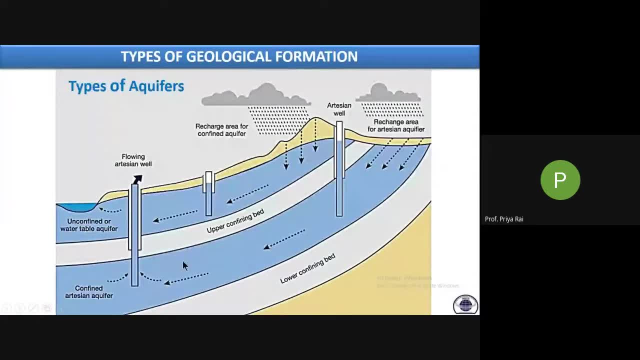 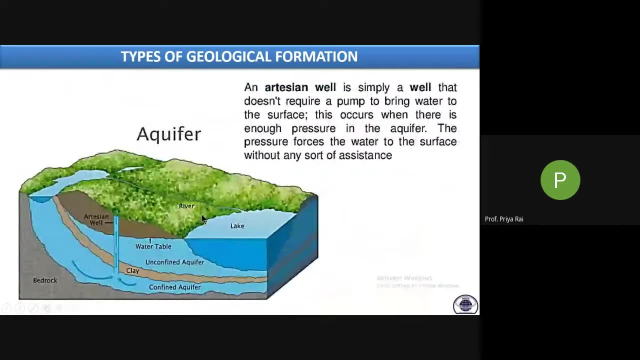 Okay, So this is your unconfined. this is your confined. Okay, Now we will show the perched aquifer in the next diagram. Okay, Look at the aquifer. One of them is the artesian well. Artesian wells do not definitely need to be dug out. 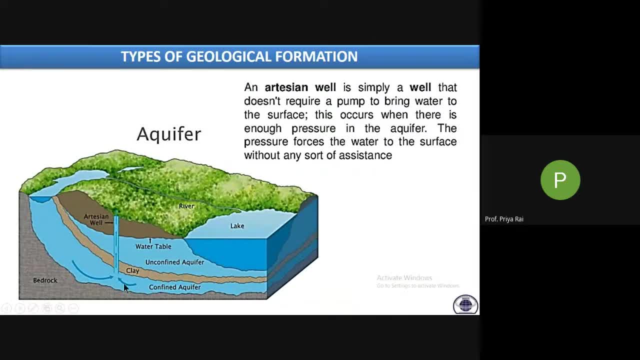 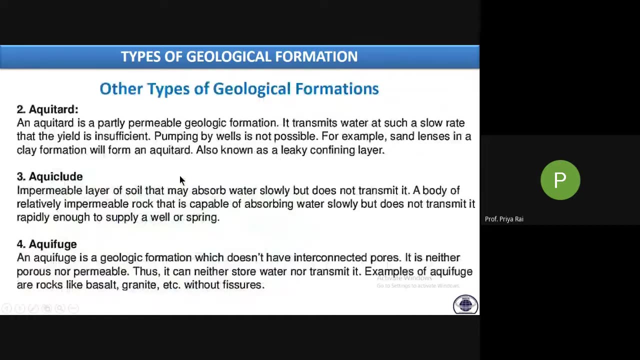 See, it does not require a pump to bring water pressure. This is called artesian well. But where is it coming from? From confined aquifer. We said that if the pressure is high, then it is coming from pressure. So this is called the artesian well. Now other types. we said 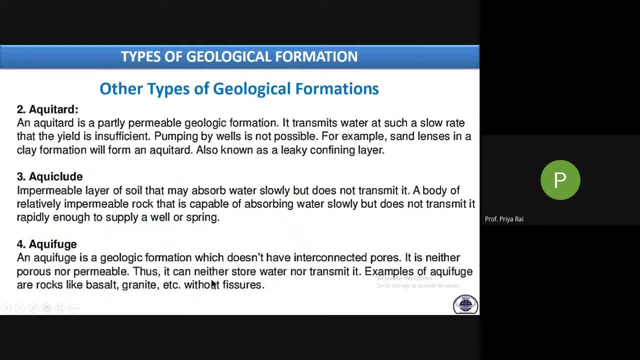 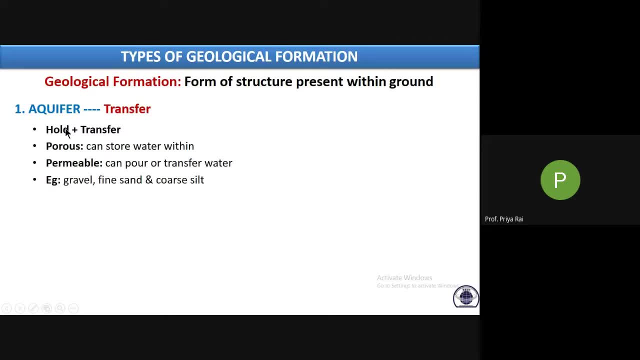 aquitard aquiclude aquifers. You have to read all these definitions Now. we will explain it in a good way. What is the hold of the aquifer? Hold means transfer. It is similar to transfer, So we will call it hold plus transfer. 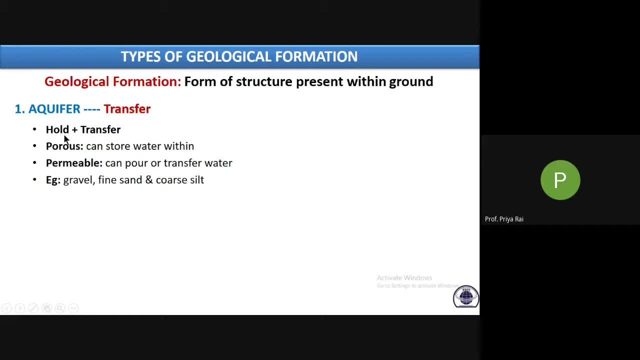 Hold means it is storing and storing water. It is also transferring. It is porous and it is permeable. also, Porous means can store water within. Permeable means can pour and transfer water. Example is gravels, fine sand or silt. 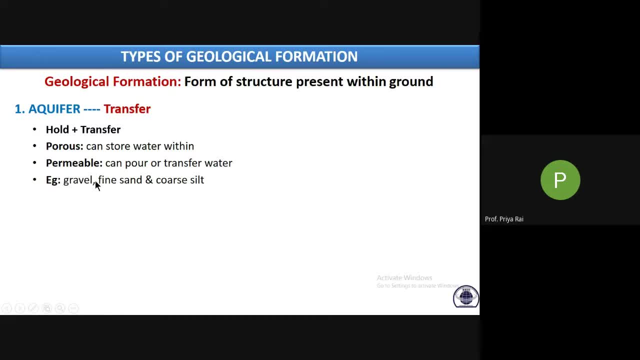 So mainly this is yours. Sand and gravel is the example, The soil structure which is made of gravel or sand. it will act as an aquifer. It means water will be stored there and water is transferred from there. also, What is aquiclude, Include- means it will. 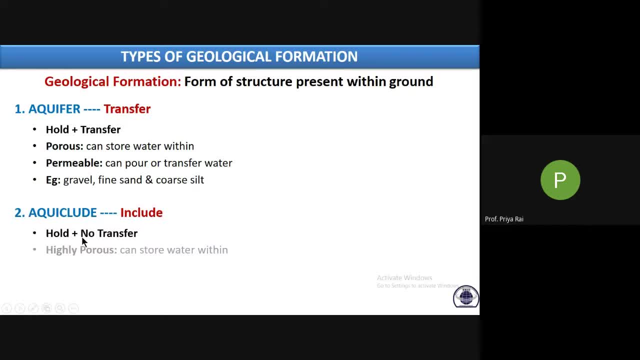 include only. It means it will only hold the water but will not transfer. So it is highly porous. It is highly porous But it is impermeable. It means it cannot pour and transfer water. Example is clay. If you take clay soil, you will take sandy soil. 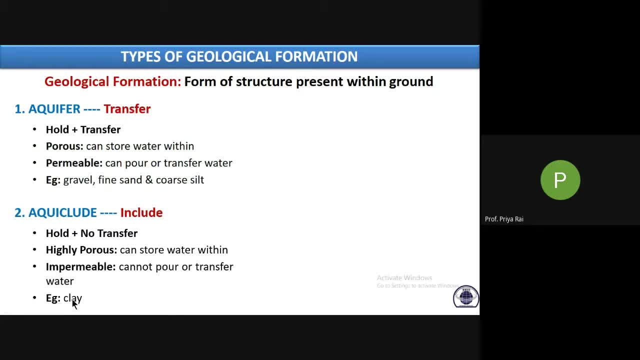 If you put water, if there is something below, if there is something like a plate with which water will drop down, it will come quickly from the sand. It will not come from clay. It will come so slowly. So why? Because it is impermeable type. 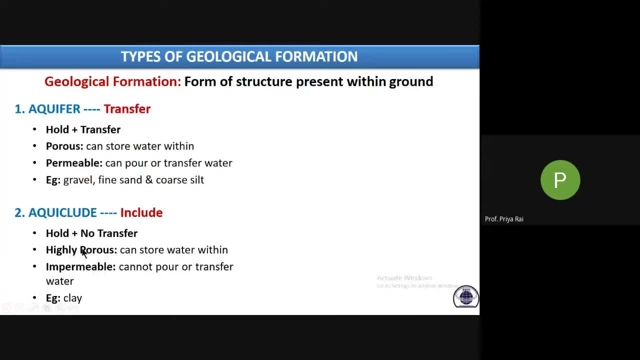 So the soil structure, which is made up of clay, will act as an aquiclude. It means it will only store the water. Aquitard is tired. It means it is a little tired. So what is this? It is hold, but it will transfer slowly. 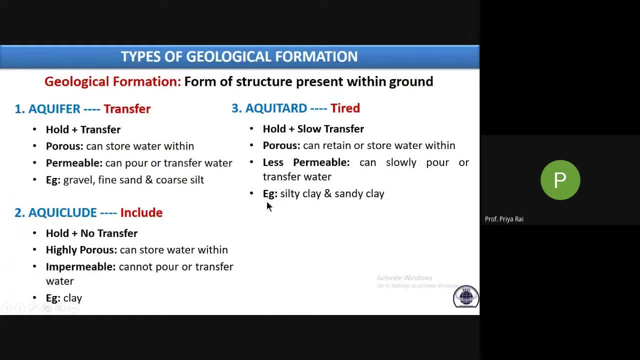 So slowly. transfer means less permeable. So what is the example? Silty clay and sandy clay. There is clay, there is silt, there is sand. So it is being transferred, but slowly. It can also be called loamy soil. 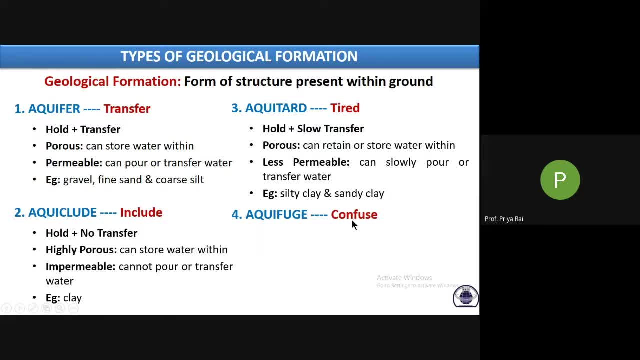 What is aquifuge? It is confused. It means what to do. Should we store it or not? So it cannot pour, neither it can transfer, So non-porous, impermeable, What is hard rock, The rocks which are there. it will act as an aquifuge. 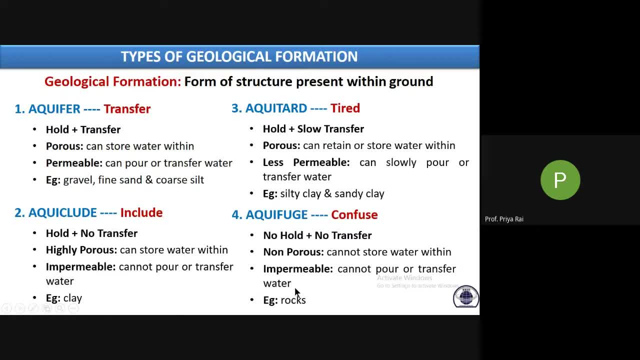 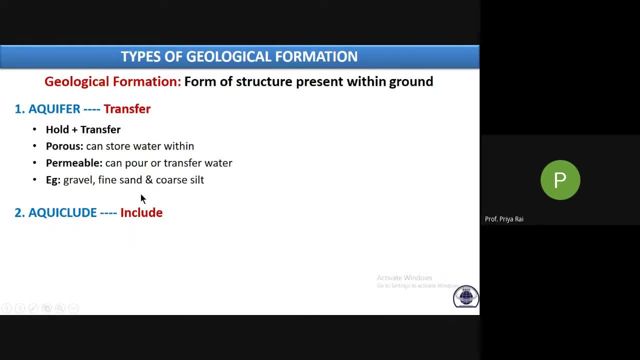 I mean, has water ever been absorbed in the rock? No, It means, even if water has been absorbed, it has been absorbed through fractures. So that is why this is an aquifuge. I think this is clear. The one given at the back. all these are the theories. 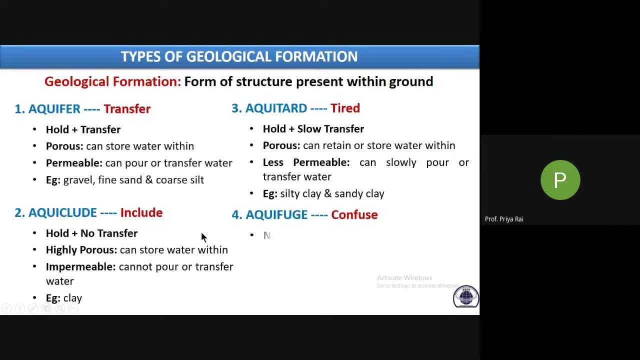 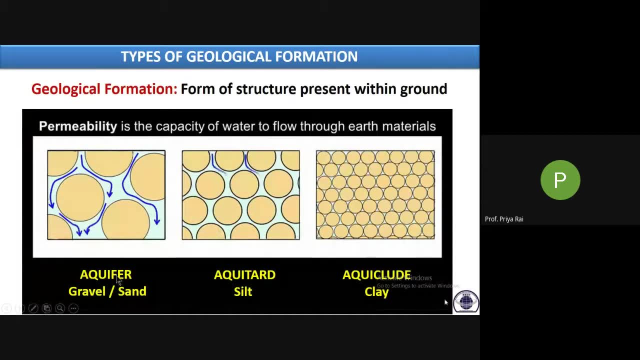 It is fine to write short notes, But remember this concept, Okay. So look, the example is this one. What is aquifuge? If we say big gravels or sand? it is permeable, highly permeable. It will flow quickly. 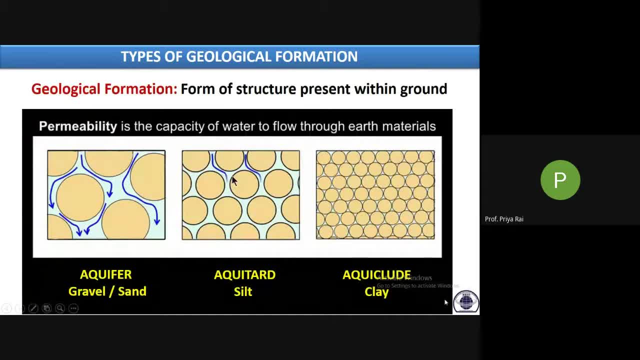 Now, what is this one? It is flowing quickly. Look at this one slowly, Because here it will transfer slowly. Aquitur retire, And this is aquiclude. Okay, So this is all clay And all three of these can hold water. 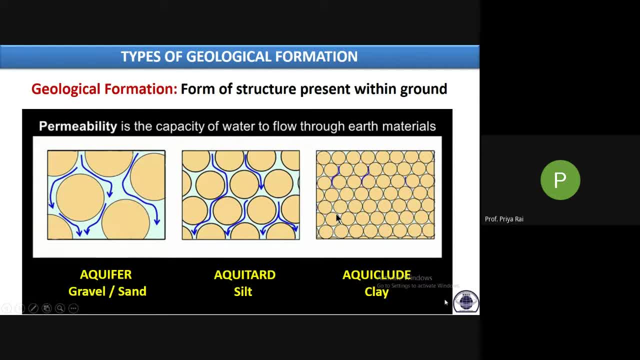 Apart from aquifuge. Aquifuge also does not hold, does not transfer. Everything holds you. This one transfers quickly, This one does not do it slowly. Okay, So look here. If this is gravel, then water is being transferred very quickly. 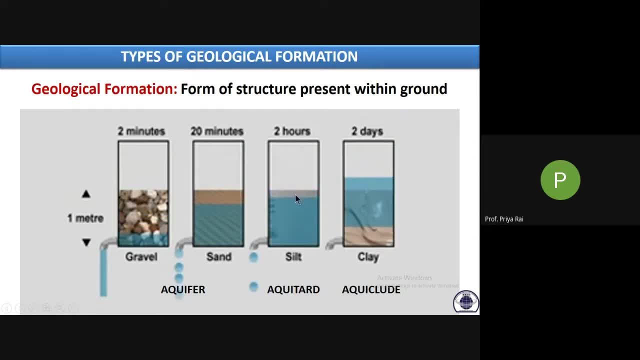 It is permeable. This one takes 20 minutes, This one takes 2 hours. Okay, So these two are an example of aquifer, Such a type of structure, Such a type of structure under the soil. So this is called aquifer. 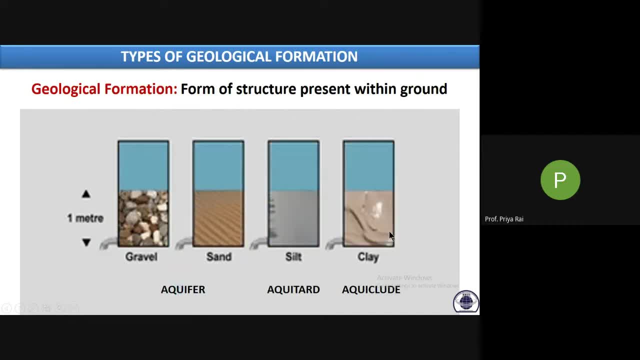 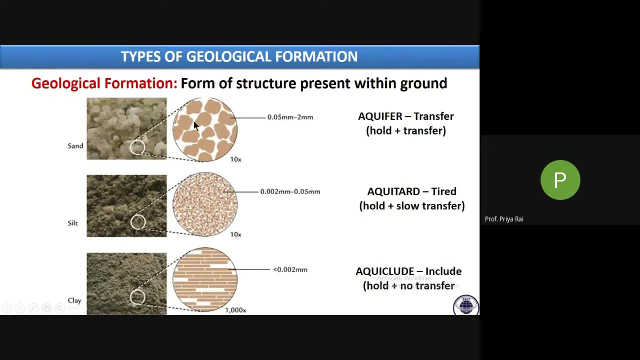 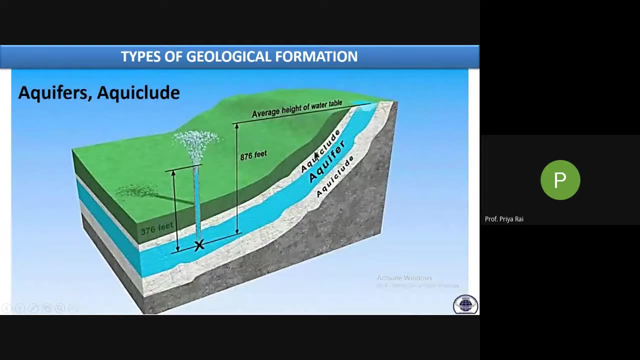 This is called aquitard And this is called aquiclude. Okay, So these are all. Look, it also depends on their structure. It is highly porous. That is why it holds, Okay. So what is aquiclude? 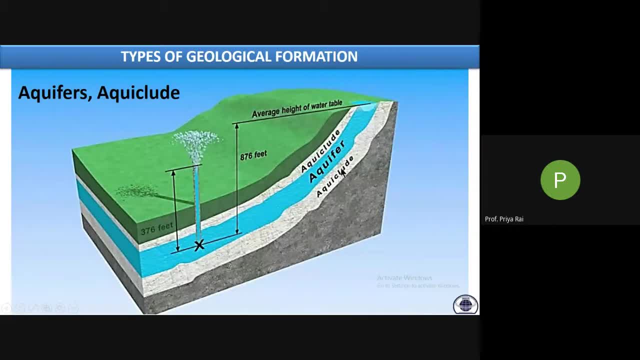 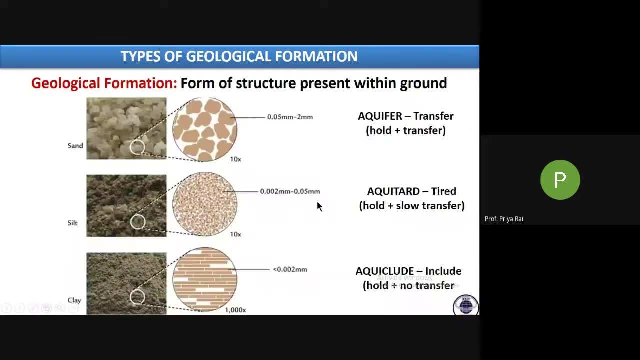 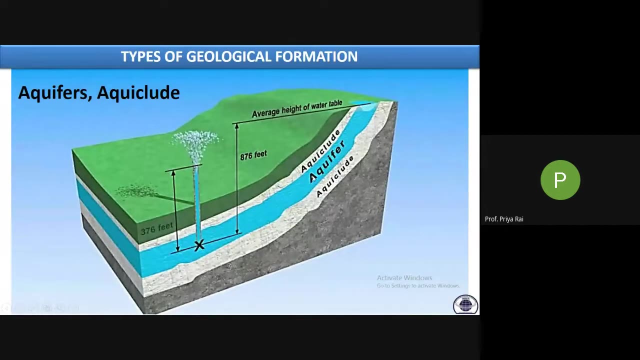 What does aquiclude mean? It does not transfer. Okay, Example is: what Example is your? What was the example of aquiclude? Clay? Okay, Clay type of soil. This is clay Clay layer. And what is this one? 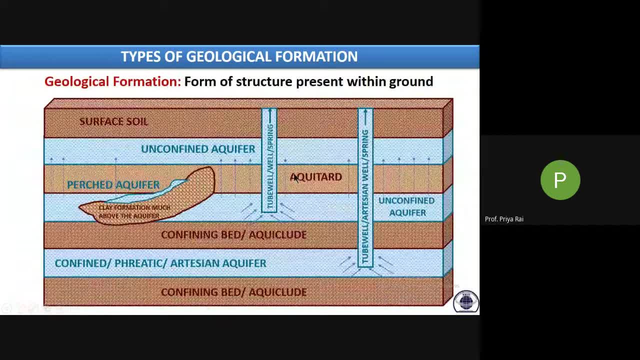 This one is your gravel or sandy type, Okay. And what is this one, Aquitard? This one is made of gravel or sandy clay, Okay. So this is unconfined Surface. soil is like impermeable: It is permeable. 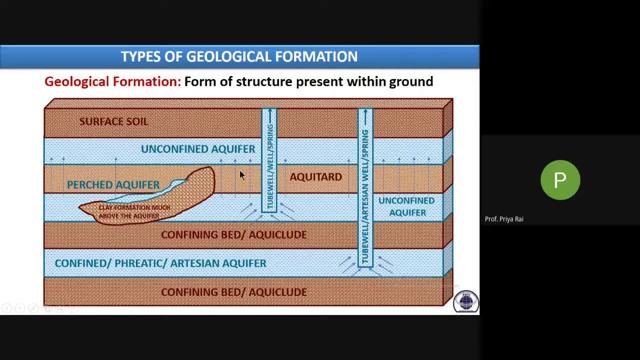 That is why the water will come down. It is like a. You can say it is permeable, Because it will transfer slowly Or impermeable. That is why it is unconfined And this one is also confined. Both are confined. 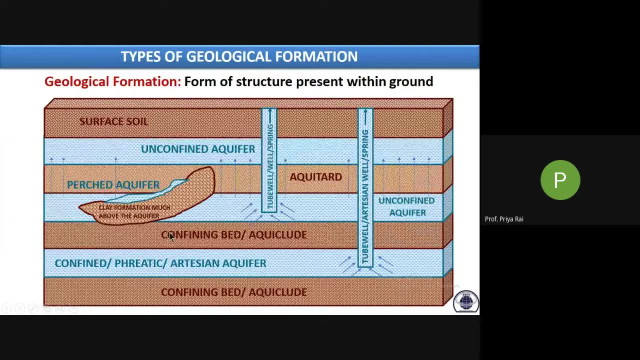 Aquiclude and aquiclude. What does it mean? It is acting like a impermeable- impermeable. So the aquifer between these two impermeable layers is called confined, Or reatic or artesian aquifer. Okay, 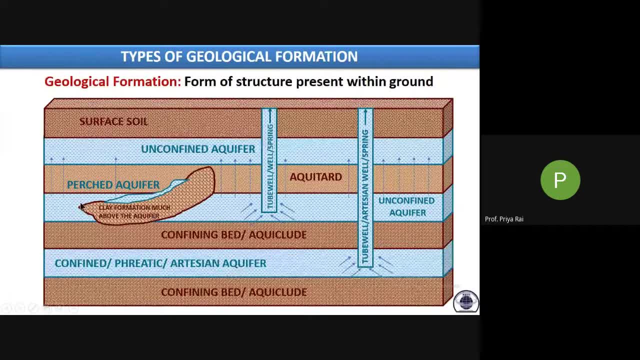 And what is purged aquifer? Suppose this is an impermeable layer, It can come, like this. Suppose there is a layer of rock in between, Like this, Water will come here and accumulate. So this aquifer is also known as purged aquifer. 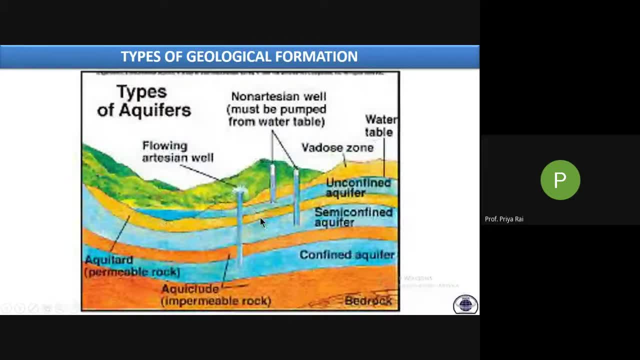 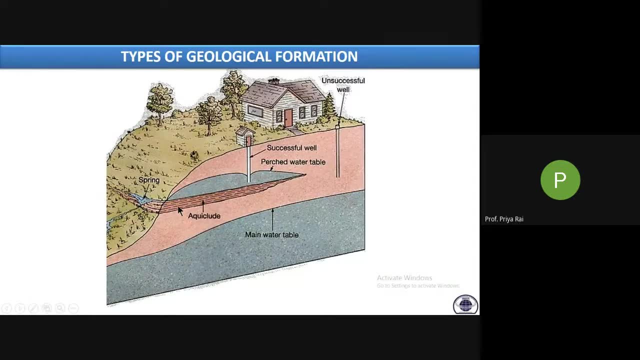 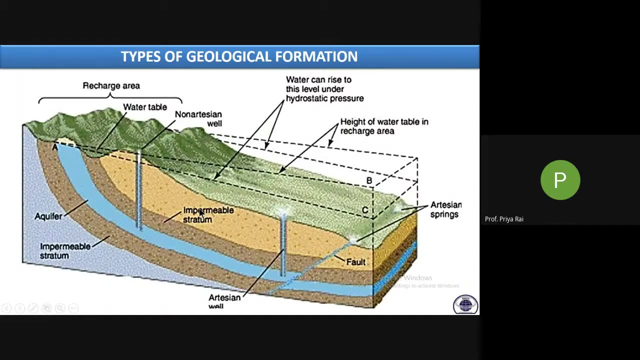 Clear. This is aquiclude. This is made of clay. It will hold, But it is not transferring the water down. Okay, So this is aquiclude. Okay, So these are the different types of formation. Geological formation: Okay. 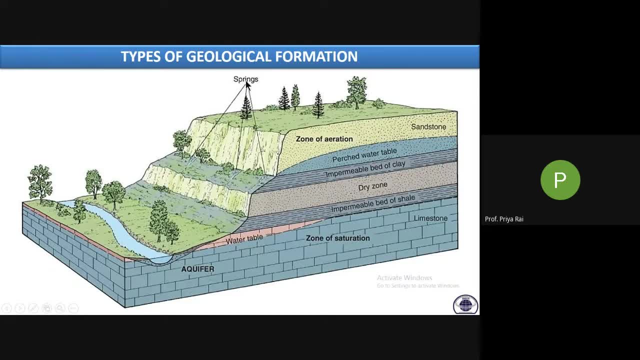 Something happens Spring. It is a natural source. It will naturally come out. Okay, It will come from the surface. You need not to construct wells, You need not to construct tube wells, Right, It will naturally come out. So it is one kind of form of utilization of geological 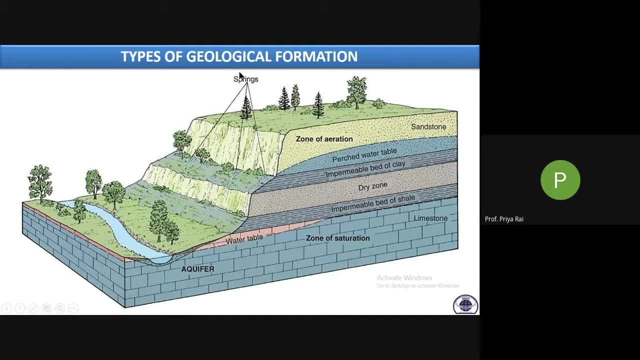 Whatever is the groundwater, How it is utilized, All this generally happens. You see, There are a lot of springs there. Spring is different. Okay, Spring is the artificial. It is naturally coming out from the ground. So, properties of aquifold. 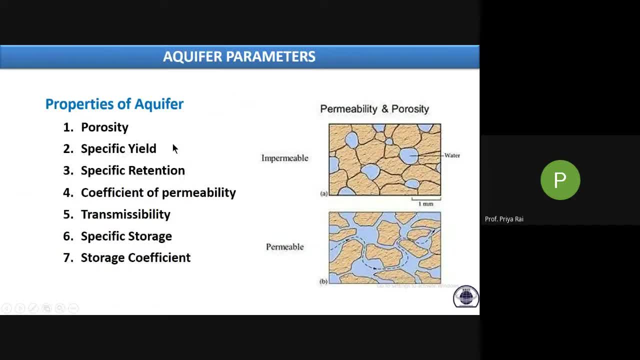 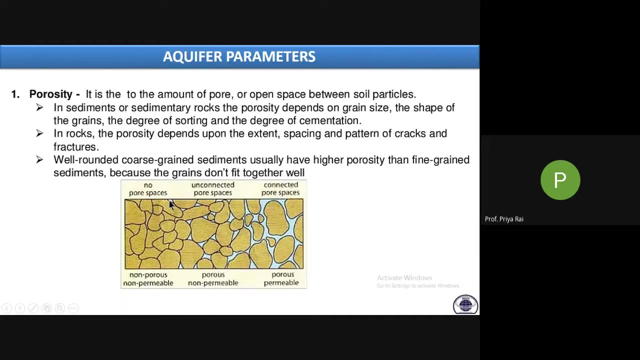 These are the properties. What should happen? Porosity, Specific yield, Specific retention, All this can come to determine in question In calculation. Okay, What is yield, What is retention? So we will see. What does porosity mean? 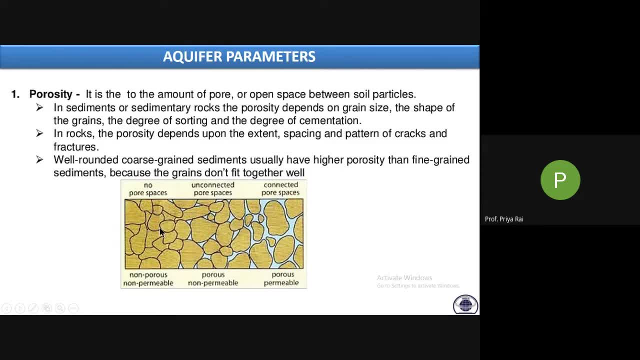 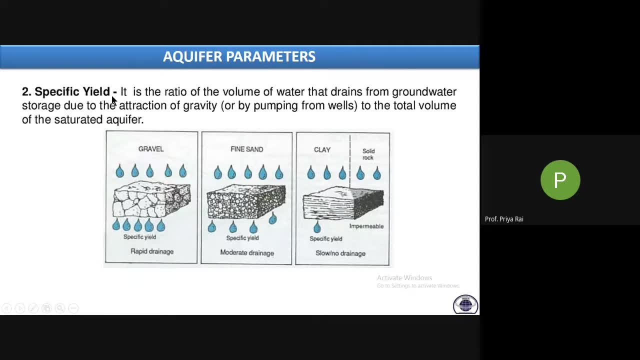 It is actually the voids. If we take total soil volume, There is a little bit here. It is highly porous. Okay, Specific yield. Specific yield means: Suppose how much amount of water That will be drained. Okay, Suppose from here. 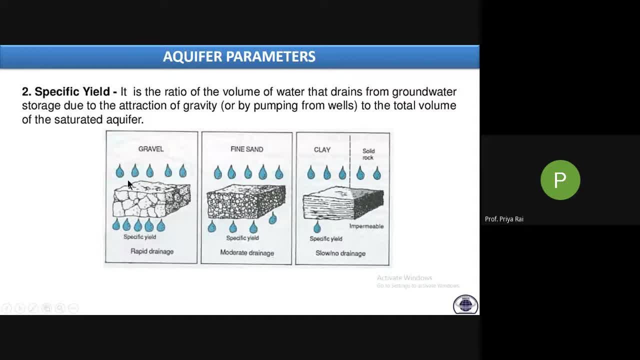 This is gravel soil. Gravel is a layer. You are putting water in it. See how much water is permeable, Because it is highly permeable. So this is the specific yield Of this type of soil: Gravel soil Fine also. 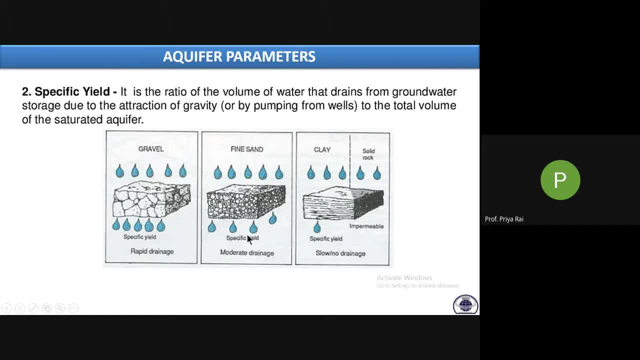 Like gravel, Specific yield A little more. But what is clay? It will not transfer water. If it does, it will do after many days. Its specific yield is very low, So it is actually the amount of the water That can be drained out by gravity. 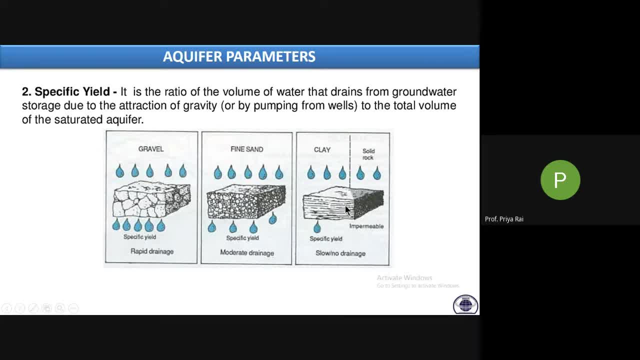 Okay. So the total volume of soil? Okay, The amount of the material. What is its ratio? The amount of the water which is drained out due to gravity? Okay, So the amount of water drained out due to gravity By the volume of the material. 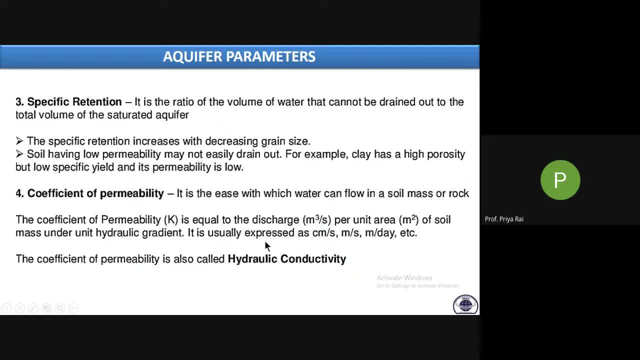 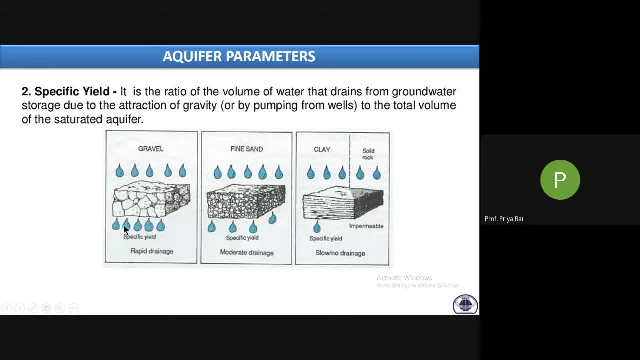 Is the specific yield. Okay, What is the specific retention? Specific retention is Not all the water will go down due to gravity. Right, Some water will retain inside. What is the specific retention Which is saved in it? Against gravity, also, something is saved. 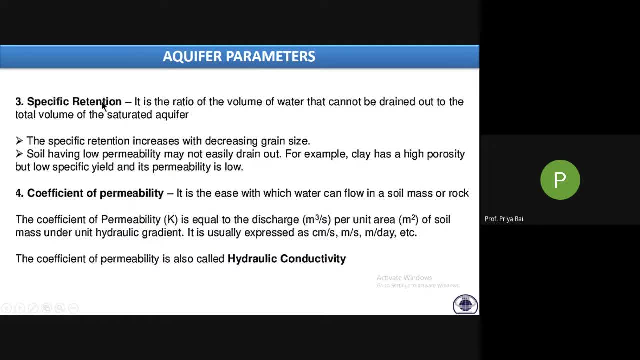 So what is that percentage? That is, the specific retention, Okay, I think- coefficient of permeability. You all are aware What is this. This is equal to the discharge per unit area Of the soil mass. Okay, Means how much amount of water has been discharged. 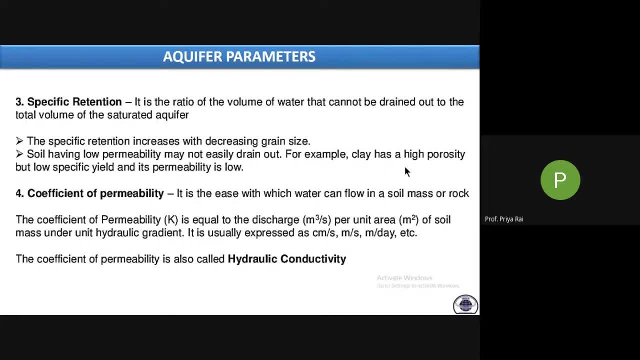 Or how much amount of the water discharge is flowing From one unit area, From one meter square area of the soil, From the soil area. Okay, So that is k divided by k. Unit is meter per second, Meter per day. Remember this unit. 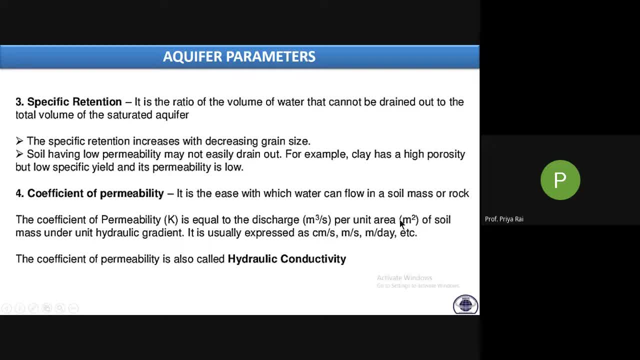 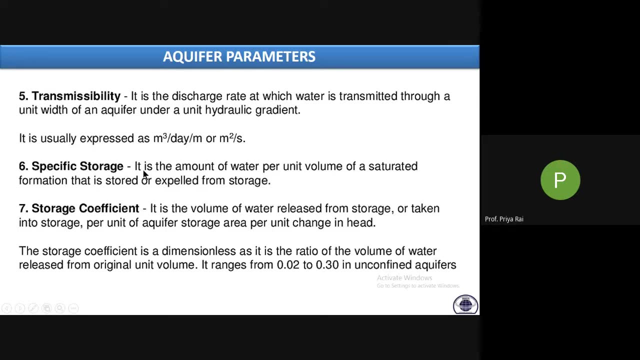 Centimeter per second, Meter per second Or meter per day? What is meter cube per second Per meter square? So meter per second, Centimeter per second Or meter per day? So this storage is what It is, the amount of the water per unit volume. 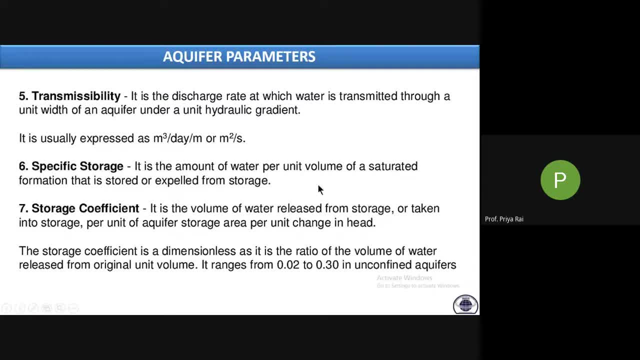 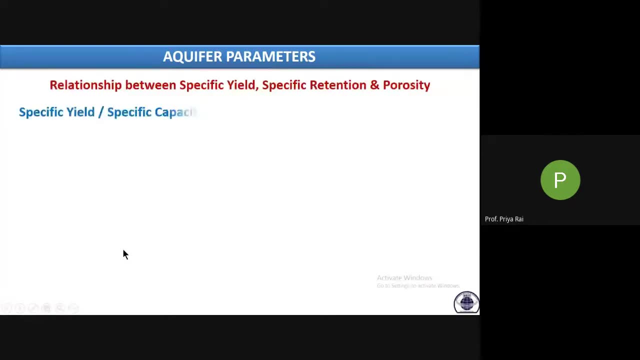 Okay, It is the amount of the water per unit. volume Of a saturated formation. Okay, Coefficient again, The volume of the water released from the storage. We will not go into all these details. When we solve the problem, Then we will discuss all these things. 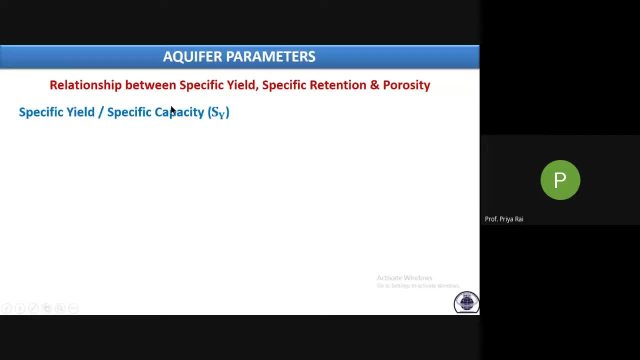 Okay, Now specific yield, Specific capacity denoted by Sy. Okay, The relationship between retention and porosity. So the first specific yield definition. As per the definition, This is your formula. Okay, What is specific yield? The amount of the water drained by the gravity. 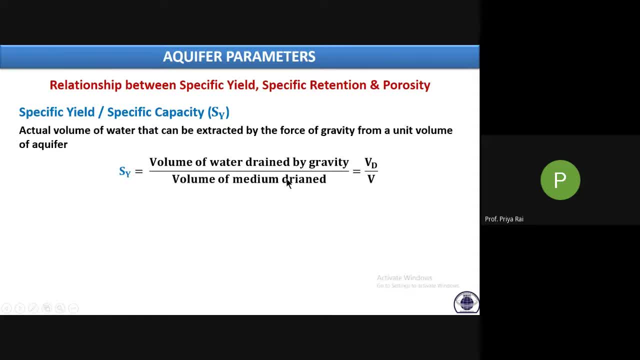 By the volume of the medium drain, Whichever amount of volume of the soil You have put water in it. Out of that, how much water went down? Take out the volume Divided by the volume of the soil particles. Okay, 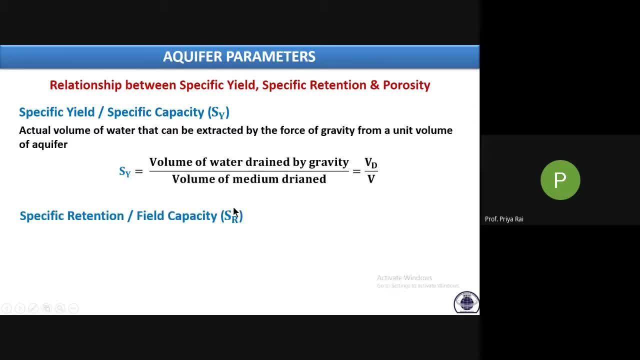 So V divided by V. R is retained. How much will it retain Against gravity? Okay, So volume of the water retained against gravity. What is this? It got drained, It went down And it survived. Okay, So Vr divided by V. 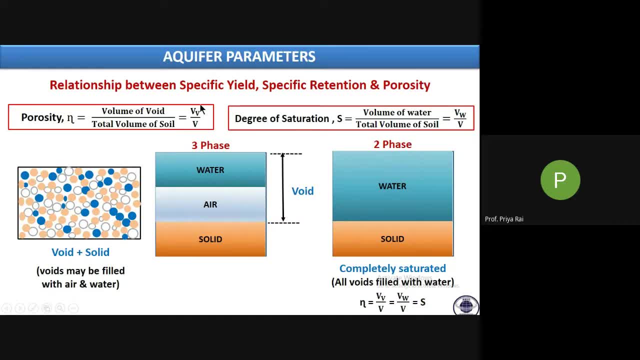 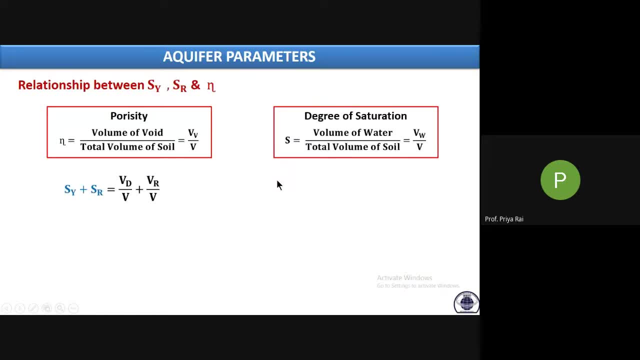 It is retained. So Vr divided by V. Now, Now comes your relationship. So see Sy plus Sr. What was it? Sy was your volume of drain By total volume. Sr was volume of retained Water retained by volume. 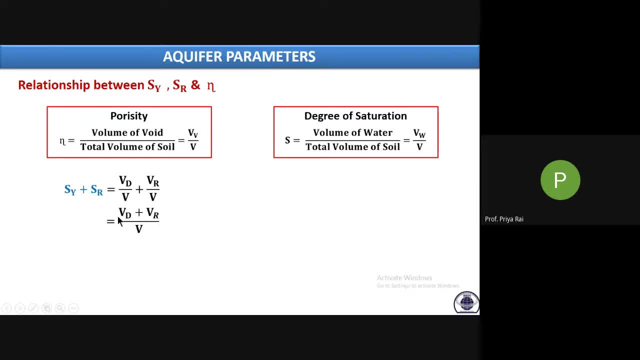 Right, So we will add this. So Vd plus Vr by V. Now see This amount of water drained Plus amount of water retained. What will happen? What should happen, What should happen: Amount of water drained Plus amount of water retained. 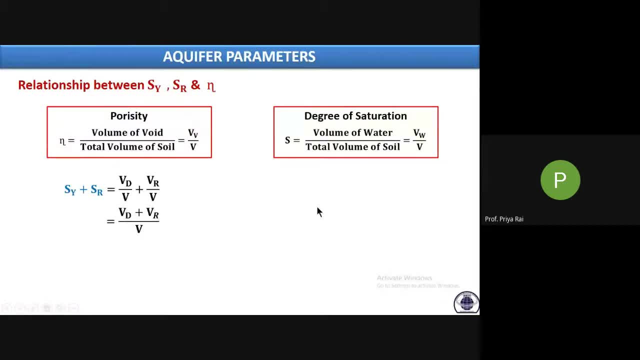 Amount of water drained Plus amount of water retained. Suppose your, Suppose, your, Suppose your Such solid particles. Okay, This is the void in between the solid particles. Okay, Some of this water is getting drained And some of the water is retained. 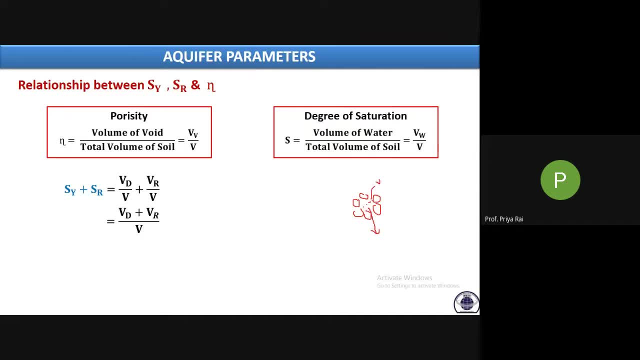 Okay, So what is here Here is Vrv And what is here Here is Vdv. So if we add these two, we will get this volume on V. Now what is this volume? These are solid particles. What is this volume? 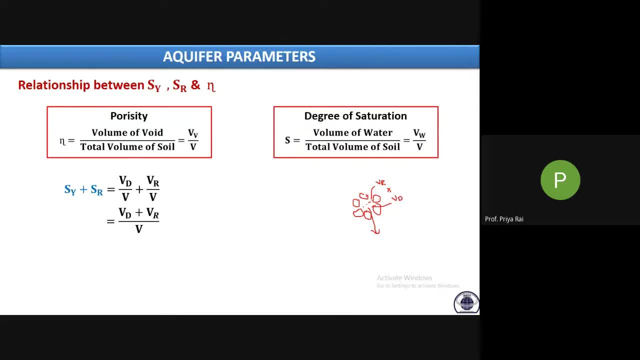 Huh, In total soil sample, solid particles remain, And what remains? Voids, Voids, Right. So this is volume of voids. So what is this? We can write Vv, Right, So see. So this is what. 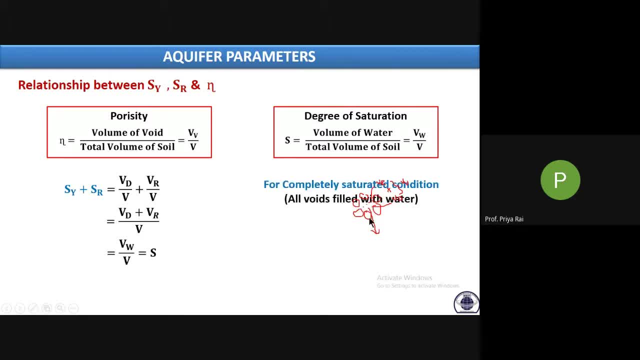 This is the total volume of water. If it is fully saturated, what will happen? We said that by being fully saturated, N will be equal to S Right, So Sy plus Sr is nothing but the Vw. What is the total water? 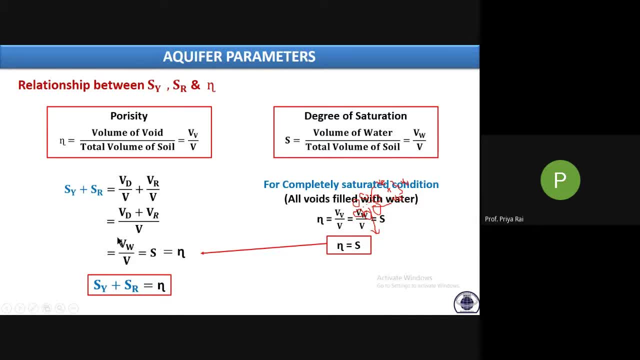 What is the volume of water? If it is fully saturated, then this volume of voids is equal to volume of water. only. That means the whole void will be filled with water. So we can write Vw as Vv, So Vv by V. 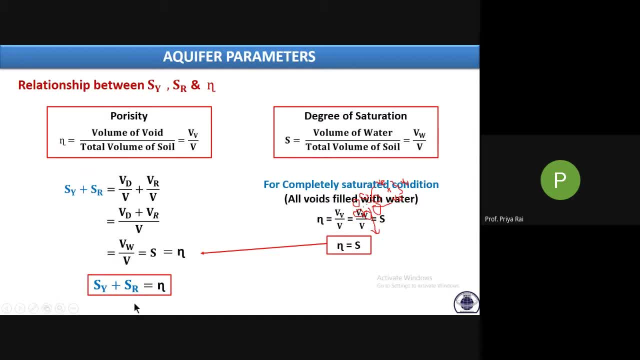 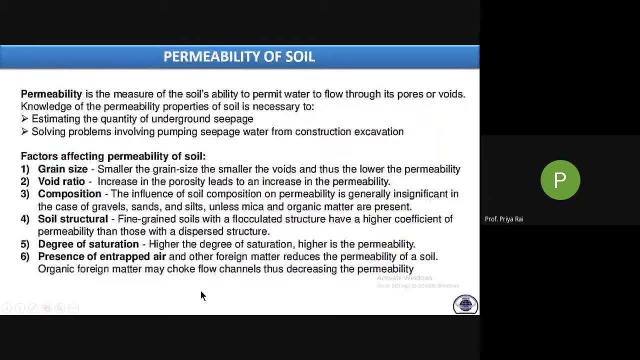 So Vv by V is porosity, So their relation is V. So Sy plus Sr is equal to porosity. Okay, This is their relation Now. next is the permeability of the soil. I mean how much amount of water it can flow through the pores. 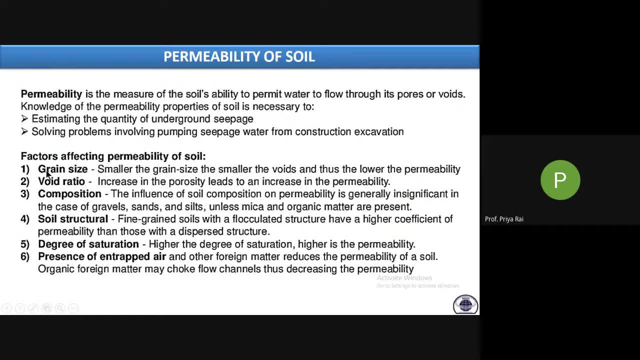 This is the permeability. Now this depends on the grain size. How much void is there in the void ratio? Okay, Porosity. What is the composition of this Types of soil? We said soil structure. Degree of saturation If it was already saturated. 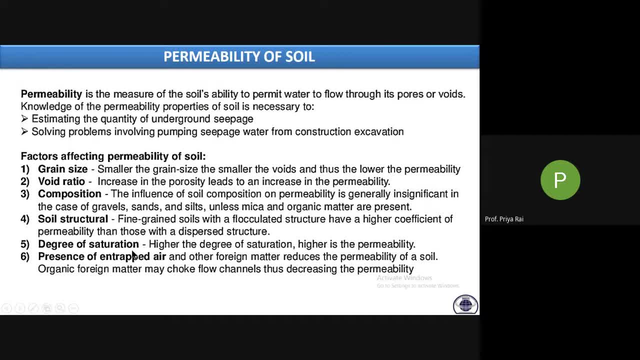 then how will it go down? What is the degree of saturation? Higher permeability: If more water is absorbed, then it will also drain out more, And again, it depends upon the type of the soil. Remember this also. So these are the different factors. 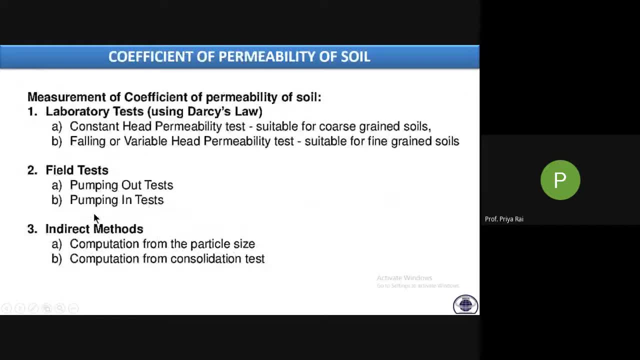 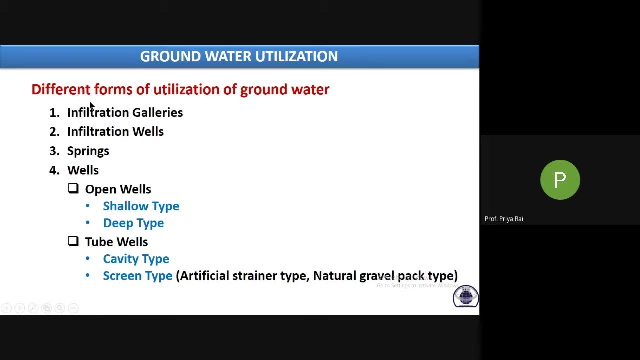 affecting the permeability. You can get these short notes Now. these are the different tests, Mainly. we will go through this now. It is not that important. Next is your groundwater utilization. What is this geological formation? In which form will there be water? 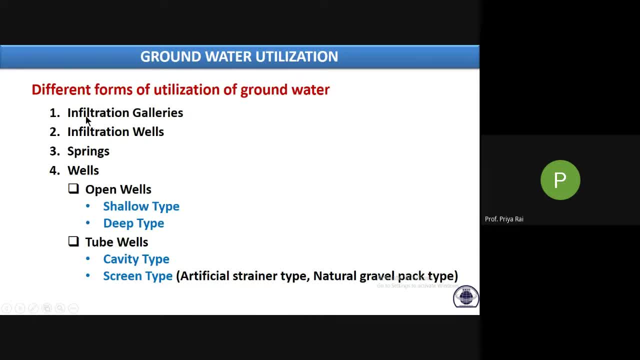 But how we can utilize, In which form we can utilize. What are the different forms? One is infiltration galleries, Infiltration, wells Springs. we said This is natural, This is artificial, But this one is natural. What comes in wells? 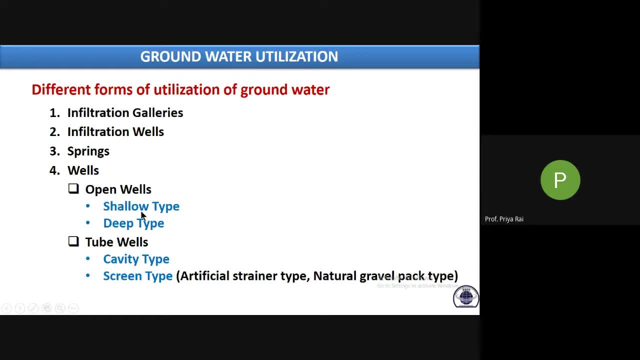 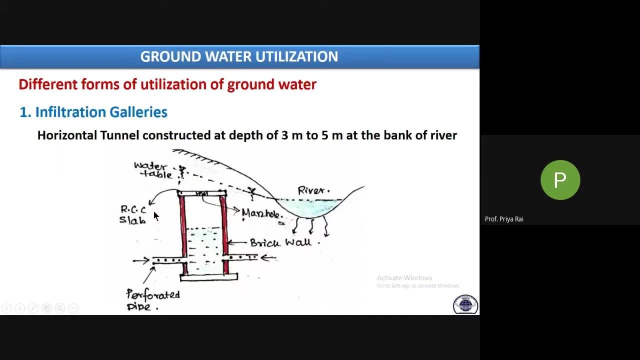 Open well tube well. Open well means well Salo type, deep type In tube. well also comes cavity type screen type. What comes in screen type? Artificial strainer or natural gravel patch strainer? Infiltration gallery is what. 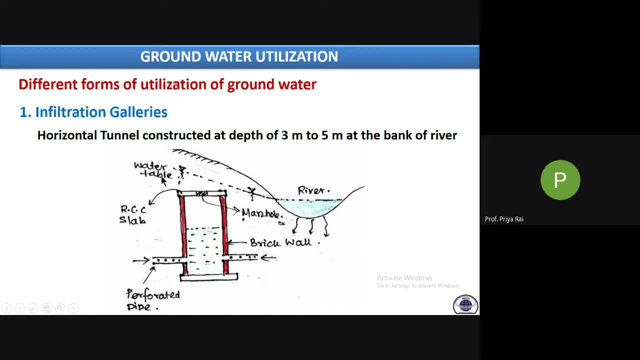 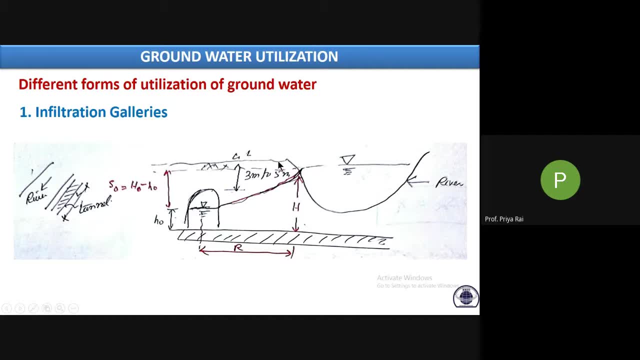 It is actually a tunnel. What does gallery mean? It is like a tunnel Like this is a river. Which is this tunnel? Some depth below? This is river cross section. Some depth below. We will construct a tunnel in this depth. 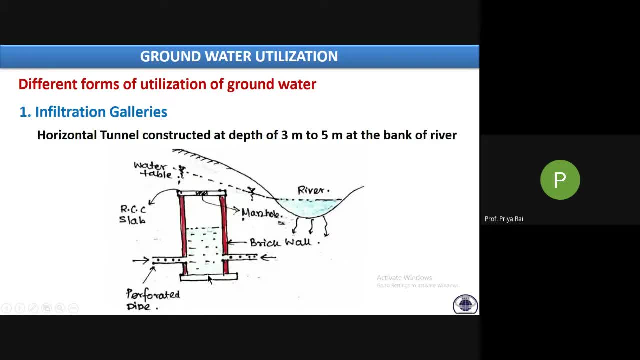 That is the infiltration gallery. This cross section view will look like this: How is water coming in this? See, this is perforated by pipe. This is why This is the ground water table. After being permeable, water will start storing here. 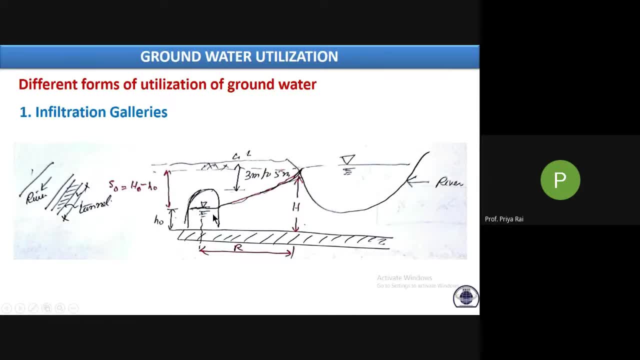 through this pipe. This is how it is storing And this is what This is the hydraulic depth of the water table. This is the depth of the water in the tunnel, And the distance between these two is denoted by R. This is H0.. 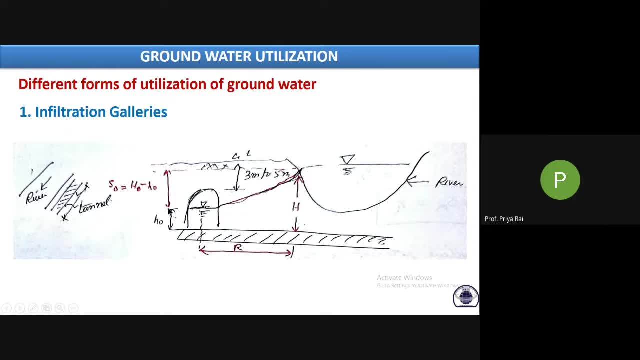 This is H. How much is your draw down? Draw down means what is the water level below this: H0.. H minus H0.. So from this you can derive that V equals to K into I. What is the value of I? 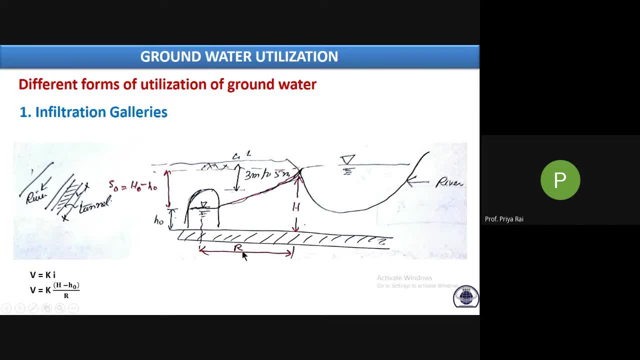 Ratio of the draw down and the distance. This is your distance. R And K is what Coefficient of permeability And Q we know, area into velocity, This is the formula of area H0 plus H by half into base, into. 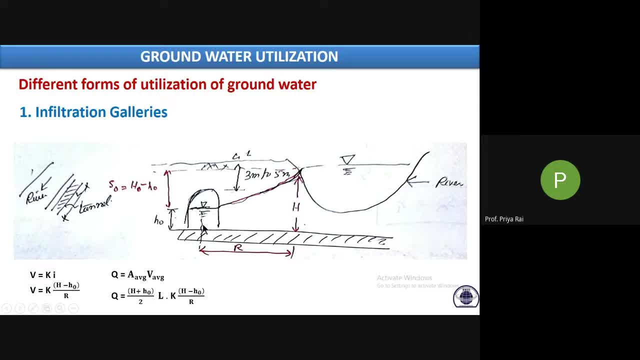 the formula of trapezoidal, So half into some of the perpendicular side, into perpendicular distance, So plus this is the value of velocity. After solving it we are getting these equations. So this is one equation for infiltration galleries. So see, this is K L. 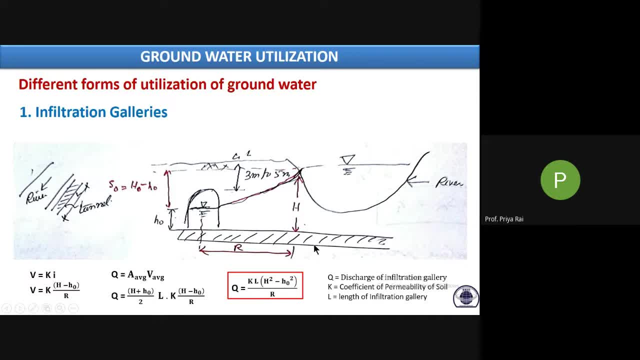 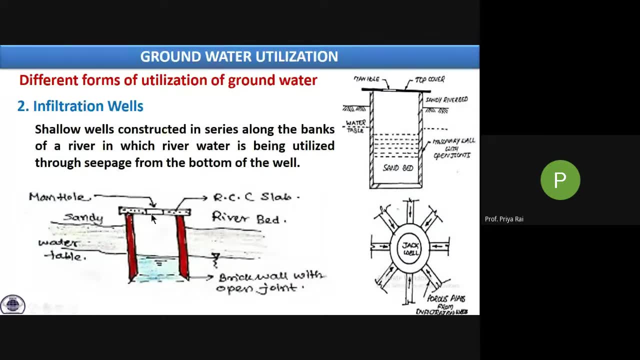 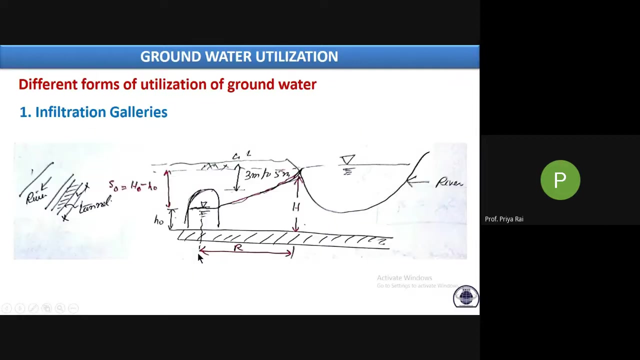 this is A square minus B square formula by R. Now what is infiltration? well, This will be: the top portion of the well should be covered and bottom should be open. Here water is coming through C-pages, You see, here, through perforated pipes. water is coming through here. 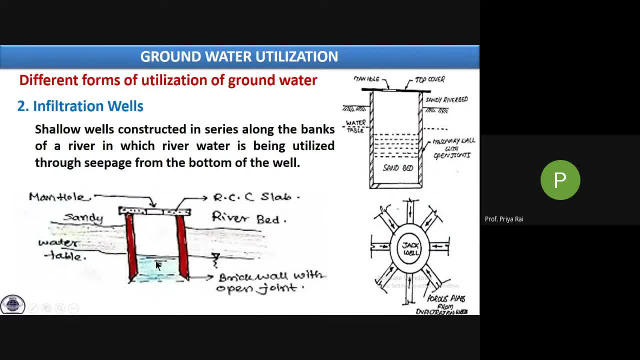 Whereas in this type of well, due to C-pages, water will be stored in this well, And actually this is the jack well, which is your main source of water. We will give a small well surrounding that, So these are what This is the main well. from here water is being stored and then stored in the main well and then stored in the jack well. 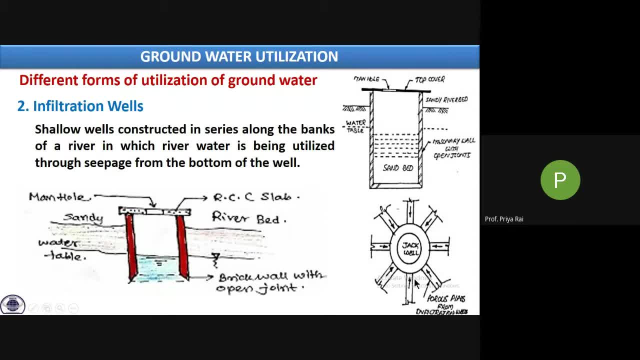 From here to here there is a well here and from here it is being stored. So these are the shallow wells, constructed in series. They are in circular shape along the bank of the river, in which river water is being utilized through seepage from the bottom. 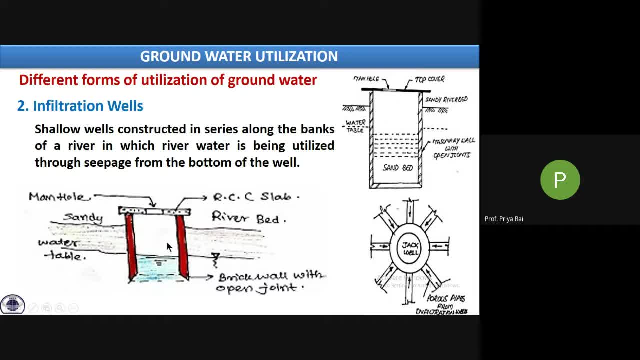 So, from here to here, ultimately, one well is like this, another well is like this, another well is like this, and everything will be stored in this, in the jack. well, We said, spring is the natural source. It is coming out naturally due to its pressure, right? 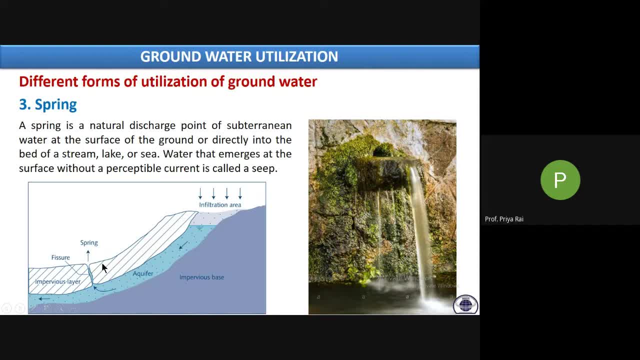 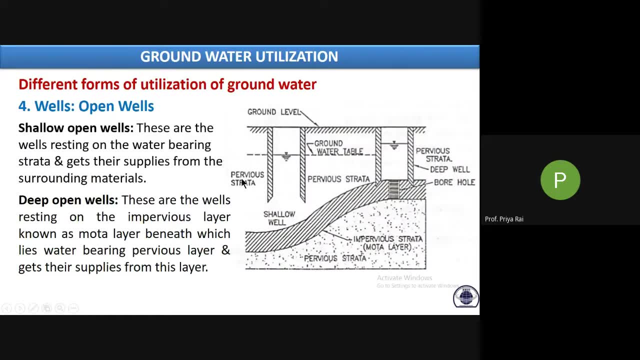 So we are not pumping it out. So artesian well is different. this spring is different. right, It is coming out through the fractures And we said there are two types of wells: Shallow well, sorry, open well and tube well. 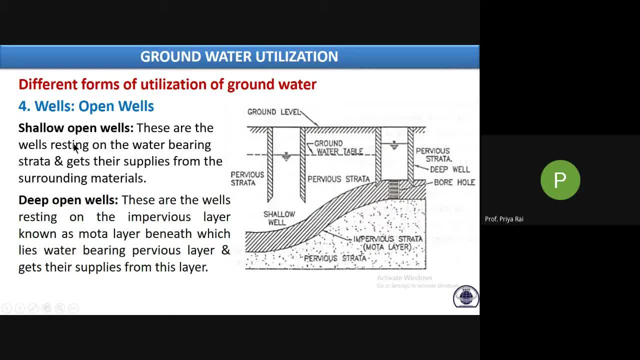 There are two types of open well, shallow, well and deep. well right, Who will we call shallow? If there is an impervious layer below, Sorry. if there is a pervious layer, Okay. And whenever in your impervious layer we dig it and get impervious layer or hard strata, which is also called thick layers? 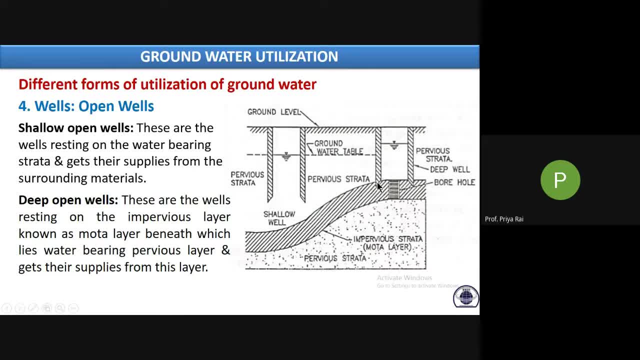 Thick layers. It ends there, its bottom. then it is called deep, well, Okay, So this is deep open, well, And this is deep open, well, See, this is your pervious strata. This is your pervious strata. 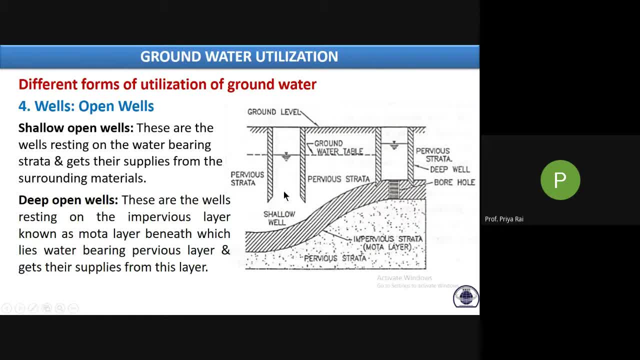 Water is being stored from here surrounding. So this is your shallow water, Shallow, well, Okay, Shallow open, well, And this is your deep open. well, What is the difference? In this, there is pervious and in this, there is impervious. 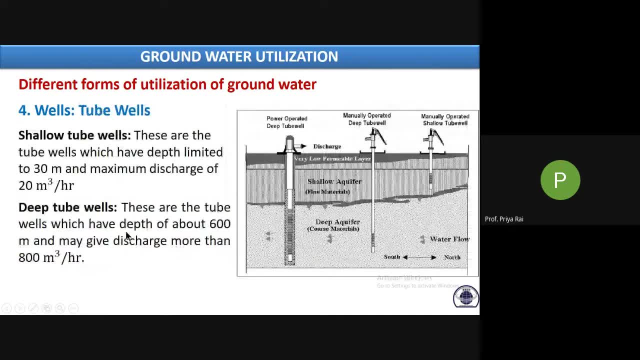 It is a hard strata. Okay, Tube well is also the same. Tube well is deep and shallow. Shallow and deep Means the depth of the well is less. The deeper it goes, the shallower it goes. The more the distance goes, the deeper it is. 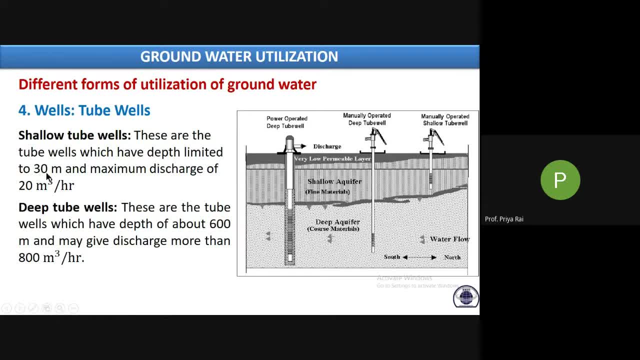 And these are some of the parameters of these people. What are the criteria? One is that if it goes up to 30 meters depth- the maximum depth of this is 30 meters- That is shallow tube. well, And how much is its discharge? 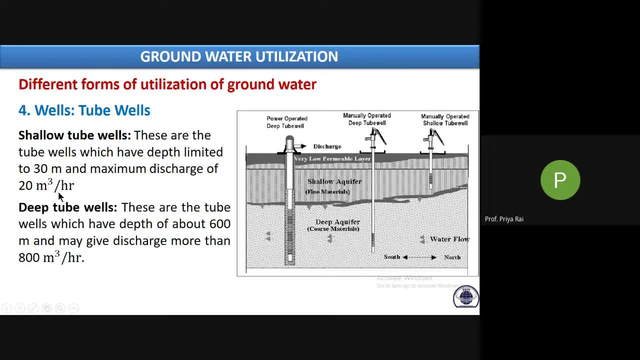 Maximum is 20 meters cube per hour. This much water will come out of here. And what is in the deep? Your depth is about 600 meters and discharge is maybe more than 800 meters cube per hour. So this is the shallow tubular, deep tubular. so this much, and we will go into more details later on how the construction is going on. 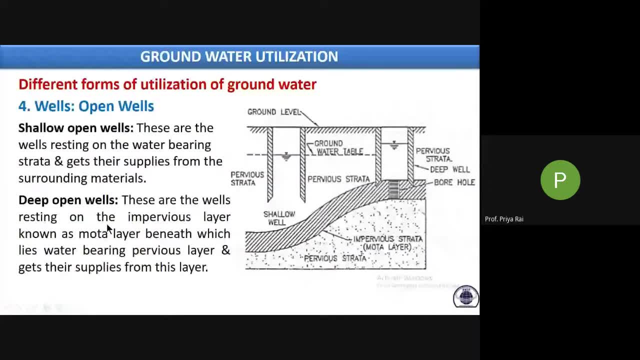 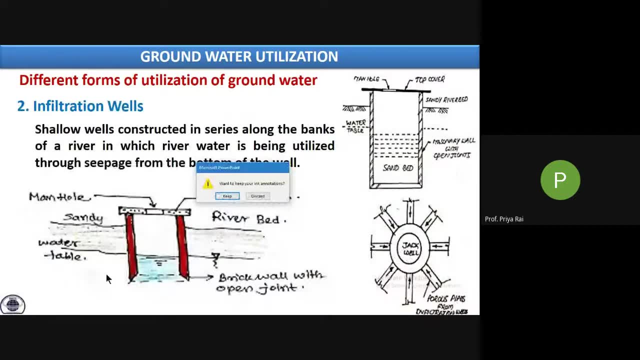 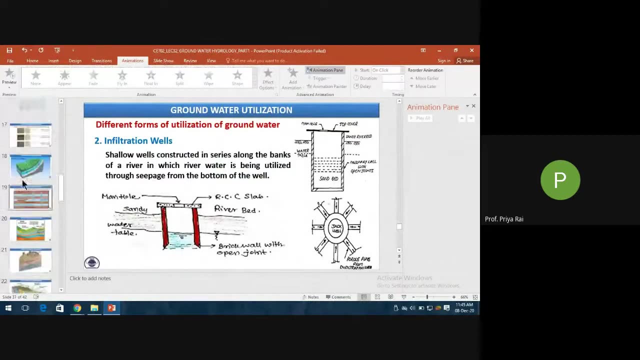 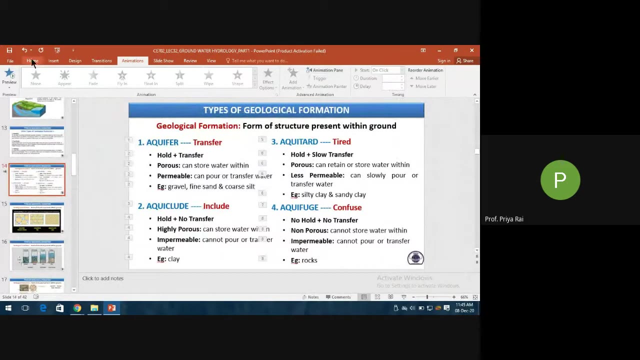 Okay, what is the time? Okay, so I think it is clear. The main topic that comes from here is this one: Geological formation. so you have to see this one, You have to see this topic. See geological formation. Okay, what is called aquifer? 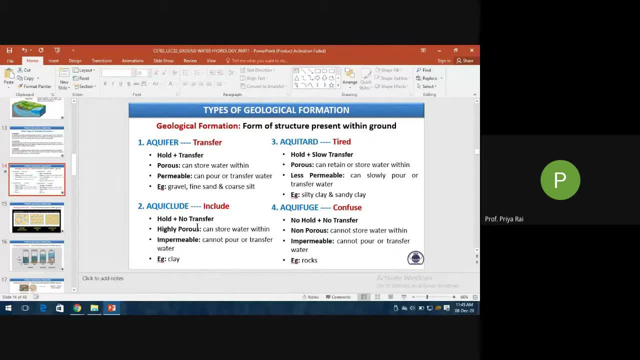 What is aquitard? These examples, along with the examples, what type of soil will we call aquifer? Okay, and this one also comes to you. What do you call it? Relationship between This one, Relationship between S-Y-S-R-N porosity? 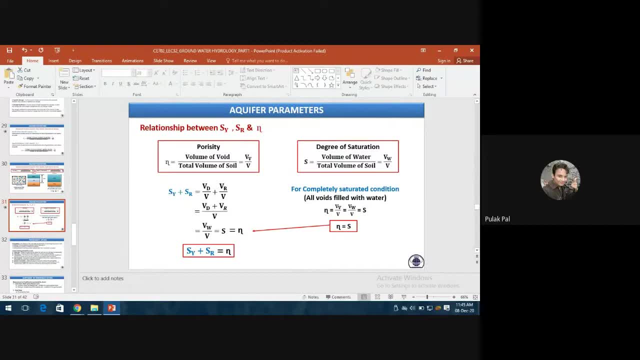 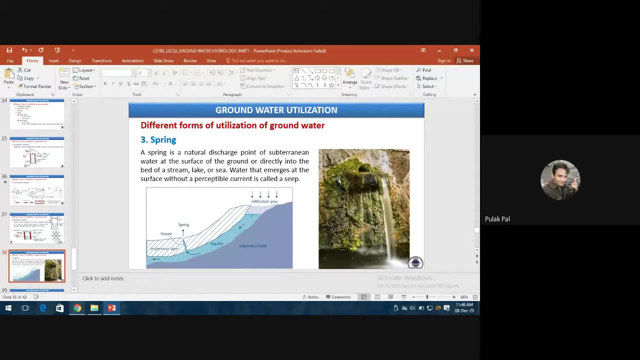 What is hot spring? What is the reason for hot spring? Hot spring, Huh, You said spring. that is not hot spring spring. Yes, yes, I understand spring, but what is hot spring? Is there any reason? I will talk about that in the next class. 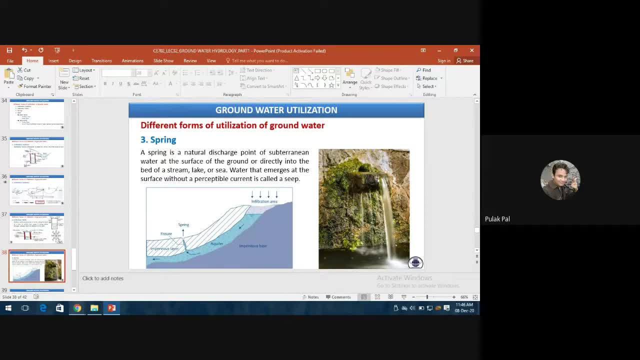 Give me some details. Okay, Spring is actually. if you see this, it is basically a waterfall. Okay, it is not a waterfall, It is a strong branch, Okay, Okay. So here in the valley, in the India valley, 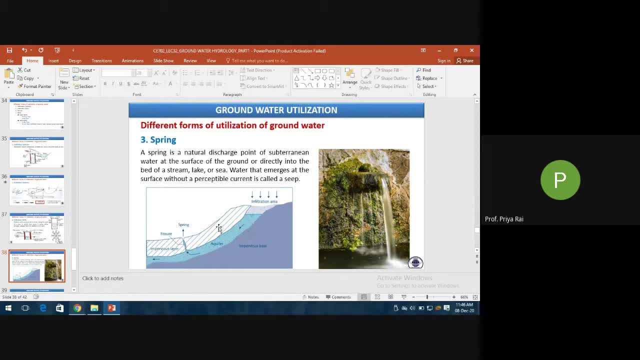 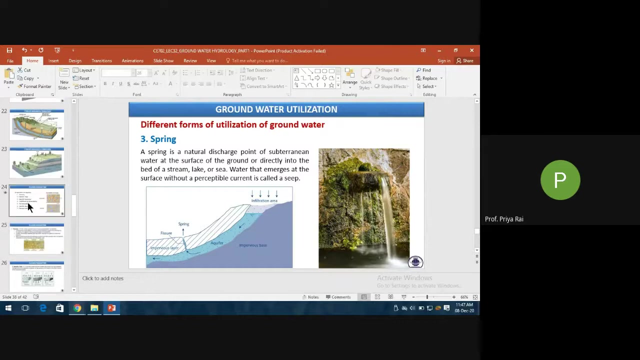 there is an article called what s buying a handsome guy? what type of guy need a? from the surface of any impervious? okay, he can watch Kelly. a thorough, a theoretical, a wallet topic for about the next classic, no problem in the dark seas laws. basically, groundwater said to.